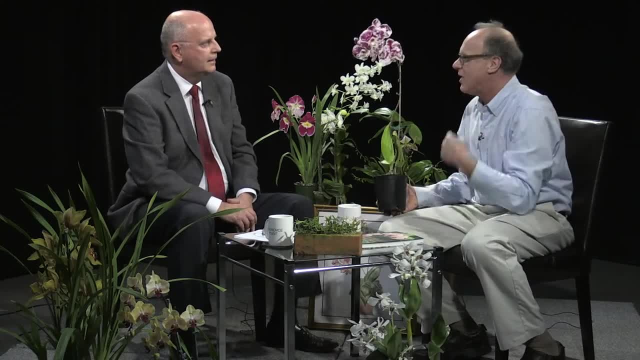 right here to start off with, even though I had to reach a little bit. This is your basic Phalaenopsis. I'm sure this is what you have at home: Basic what? Phalaenopsis? Phalaenopsis, And there's a. 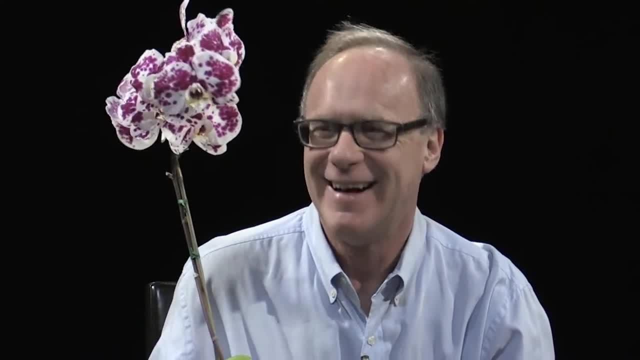 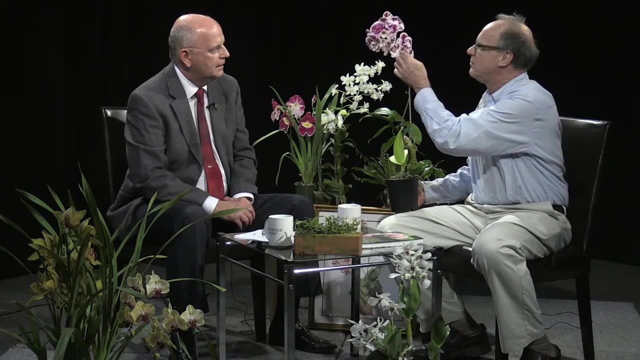 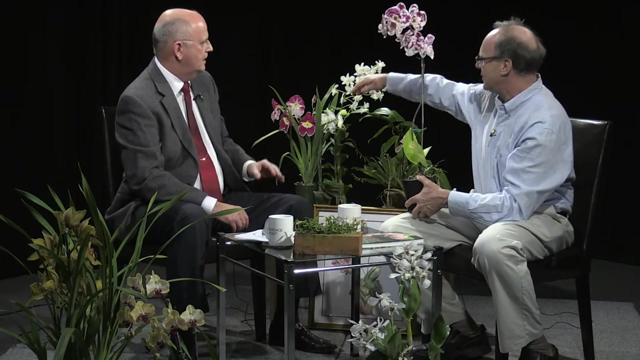 little cute joke that goes around: You can't fail with a fail. but people do fail with fails and it's easy to do because they don't necessarily bloom back automatically. But here's a little trick right off the bat. And are there different colors? Yeah, you see, here's one with white, with red, and then there's a pure white one, If you look. 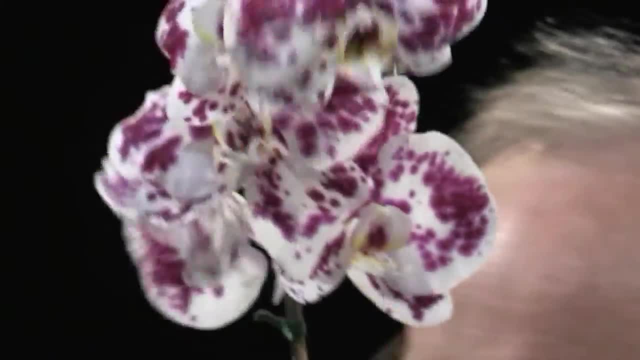 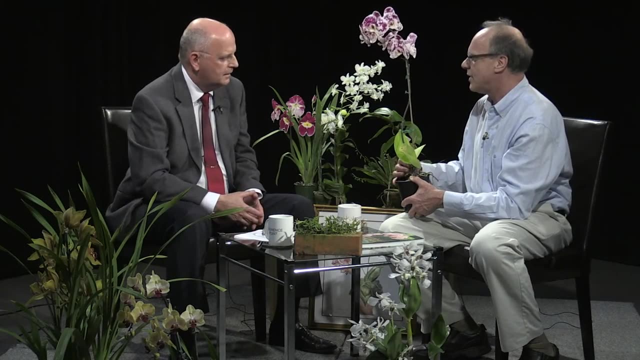 closer on the door there's one with the little yellow. They come in all different colors and they all have the same little leaf like this, the leaves like this, And they're called monopodial in growth. In fact, the growth is only directed in one direction, So it's called 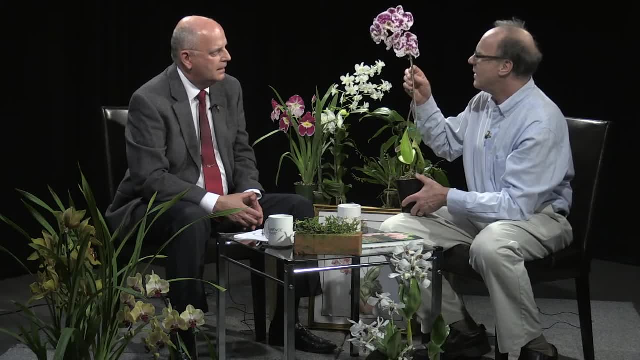 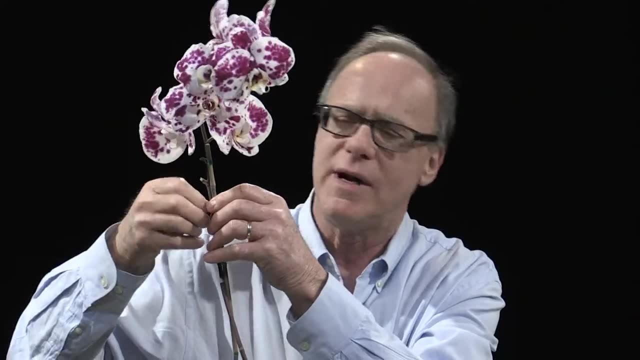 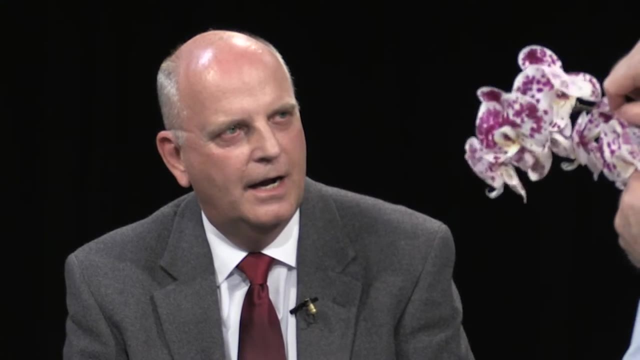 monopodial growth. Now, with these you can do an awful lot, because I mentioned to you earlier that I worked for, like Ralph Lauren Polo at one point. Well, if you wanted to, he wanted. this was 25 years ago and they wanted to get an orchid with a certain kind of bend in it And you can take a wire and bend this and bend. 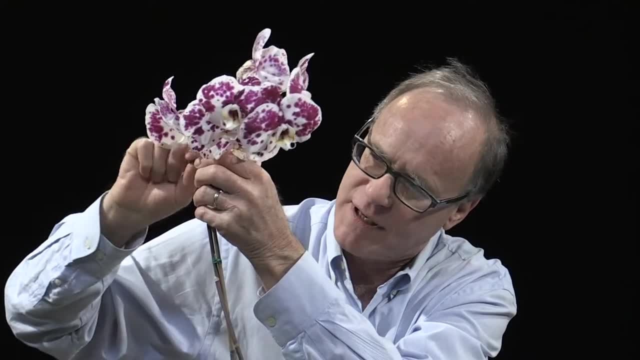 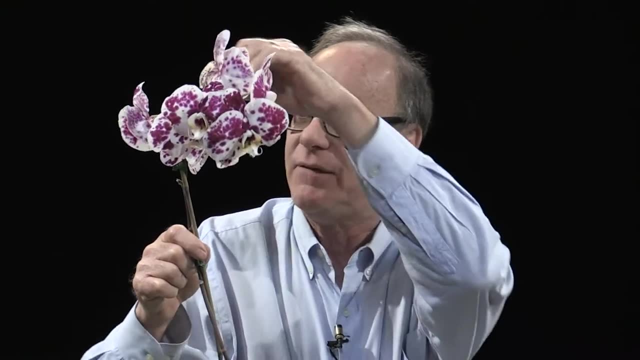 this stem and rewire it, and you can. you could force it in any kind of any kind of angle you'd like to. So there's a little. there's little tricks all about. all about what you do with these little orchids If these orchid flowers are starting to die, like at your house, and you're getting down. 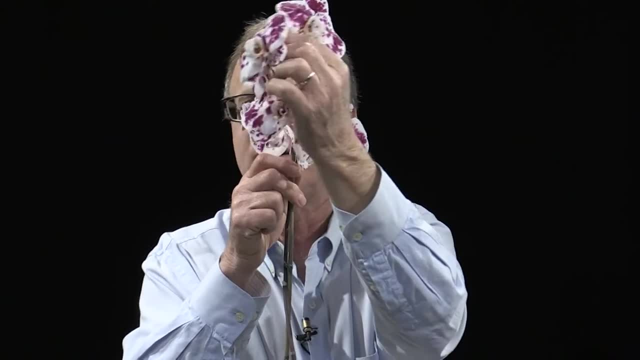 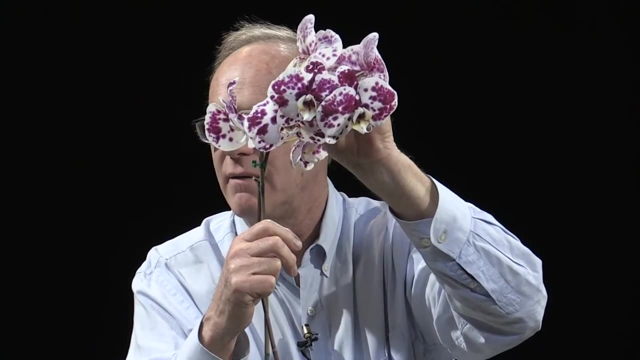 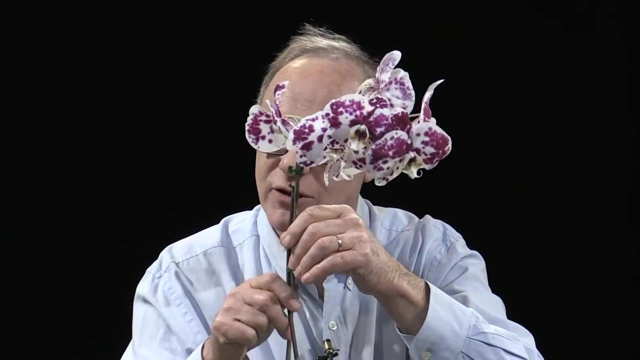 the last one or two flowers before this very last little flower at the very edge of this stem dies. just count back one, two, three flowers and break the stem there and that'll send out another stem from the same branching, from the main stem. and oftentimes when you go into flower shops you see 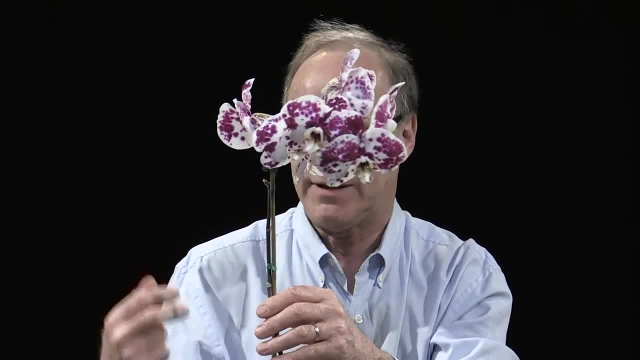 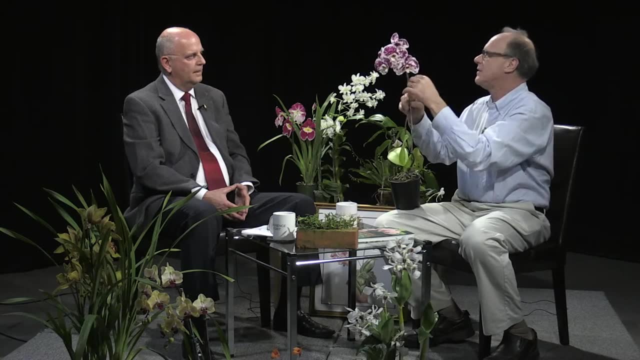 all these these phalaenopsis, and they'll have two and three and four spikes coming up. okay, and that's how people do it: They've cut down, they've, they've blinded the the end of the stem, and then the new branches have indeed come out. So if you let it go all the way until the last blossom falls off, it's. 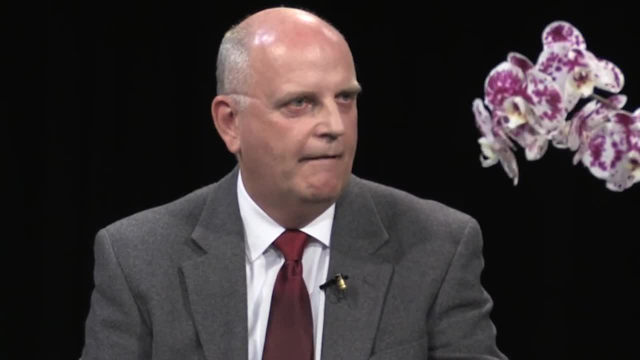 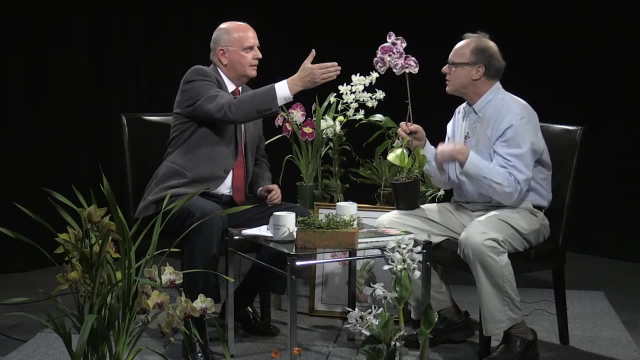 going to be problematic whether it's going to re-blossom again Exactly at that point. the stem usually turns brown and then you just end up cutting off the stem. But if you go back, you said the as long as there's some life left in the flowers, just cut, just count back from the very end. one: 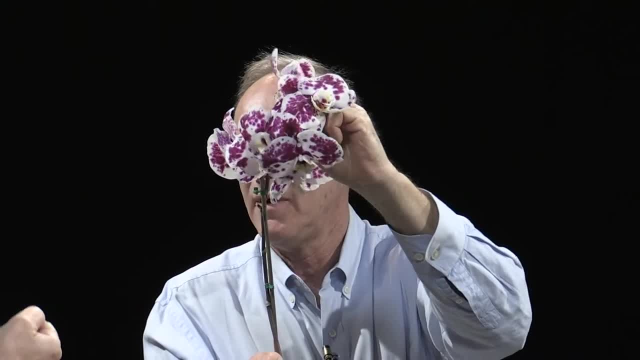 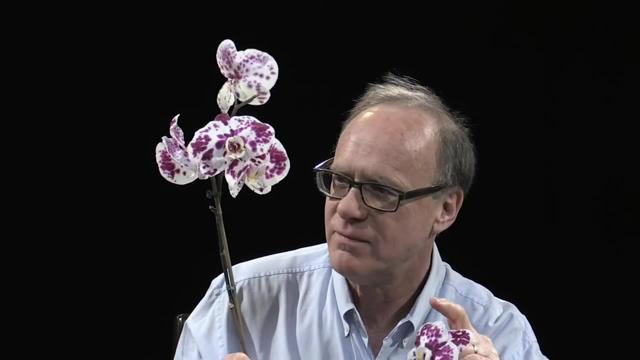 two, three flowers. give it a little snip. uh-huh, I'll do it right now. leave a little snip like this: I want two flowers, I'll go one more and what's going to happen here? you could wear these and you lapel later on this evening. We'll keep you busy tonight in the, in the social, social areas. 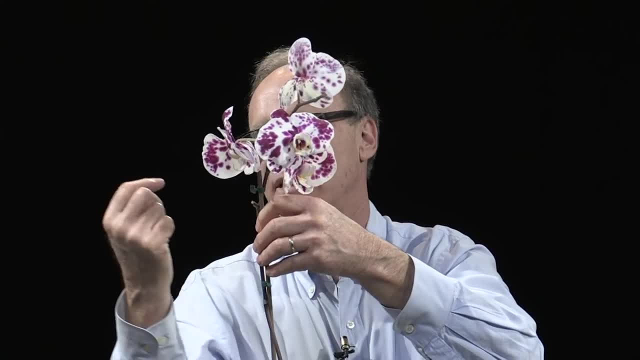 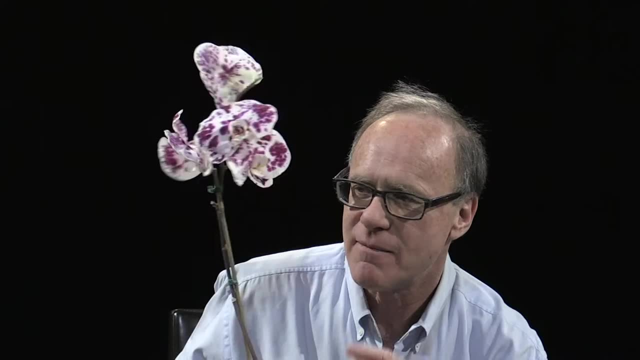 and then what will happen here is right about here. you'll see a new branch coming in form before these will die, And so that's that's how they do it Now. does that work with the virtually all orchids? No, we're just talking about Phalaenopsis here, Just with Phalaenopsis. 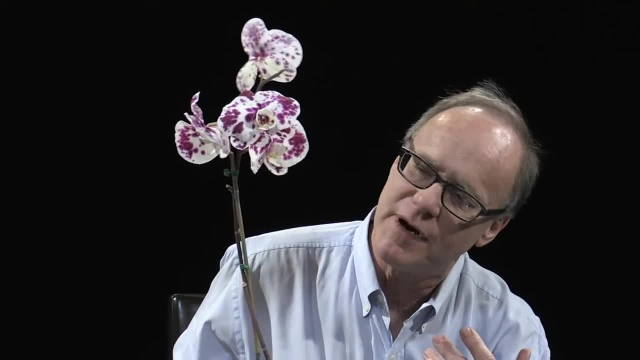 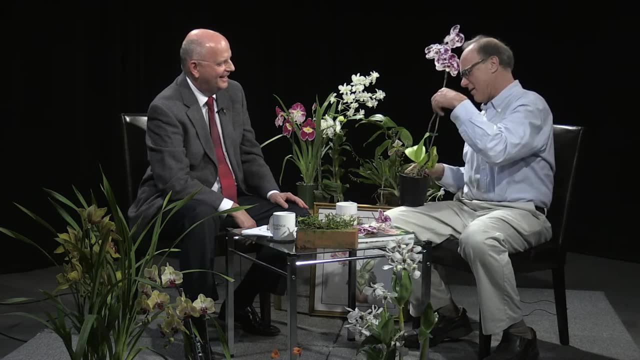 And with Phalaenopsis there's a lot of tricks you can do, like, for example, if you have some that have never bloomed back. they're at your house every day, probably in your bathroom or your living room, looking ugly because there's no flowers. not just have these ugly leaves sitting here. 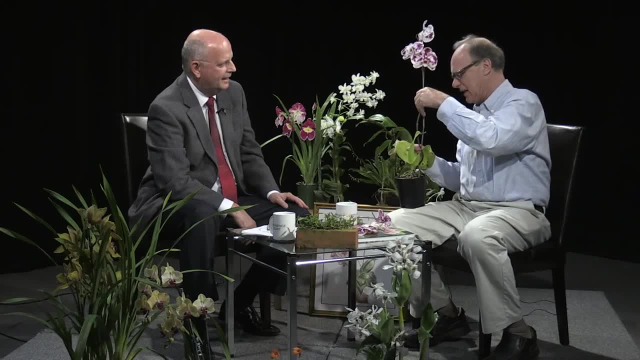 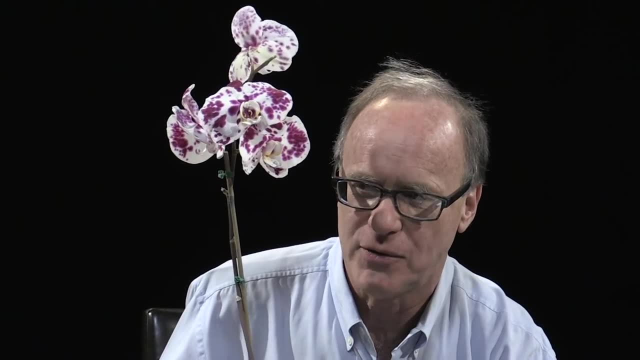 and no one really understands decorating wise. what's going on? it's ugly, it's ugly. well, listen, just take that plant and if you live like in the bay area, you can either throw it outside on a cooler evening, overnight, just for one night, or you can even throw it in the 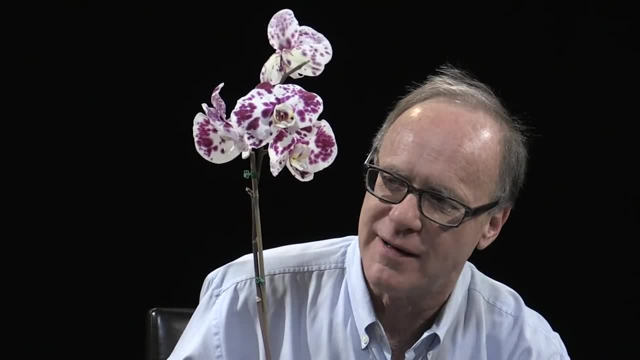 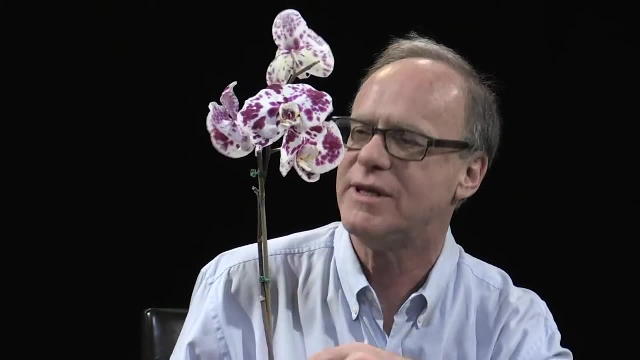 little salad bin in your refrigerator and sometimes that little cold snap will. it'll trigger exactly, and then then about a week later you'll see a new stem coming up. so if I go into a flower store or go to a place, because you see them, all kinds of places, you'll see them. 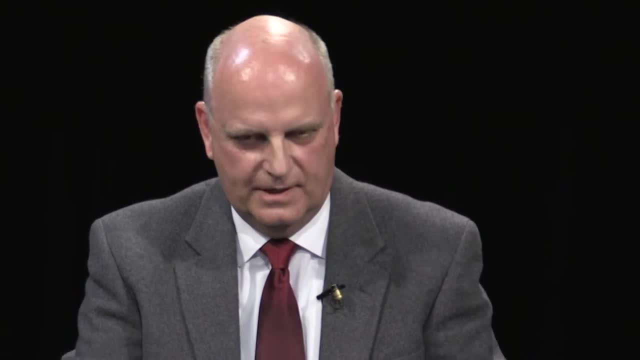 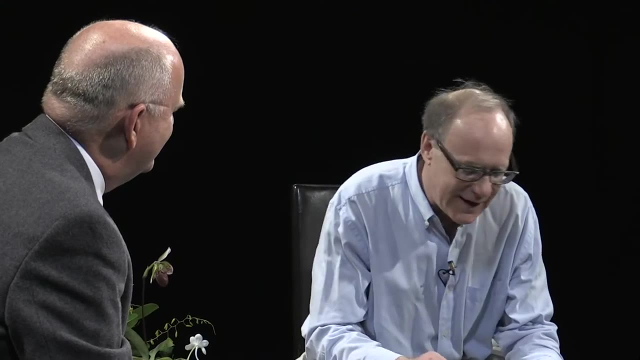 at even that, the the flower section of places like Safeways or whatever Absolutely Tra Drive shops. Will it say Phalaenopsis On it? how would I know that that's what I'm getting? Well, these, you'll have to learn one orchid this afternoon, because that would kill you. 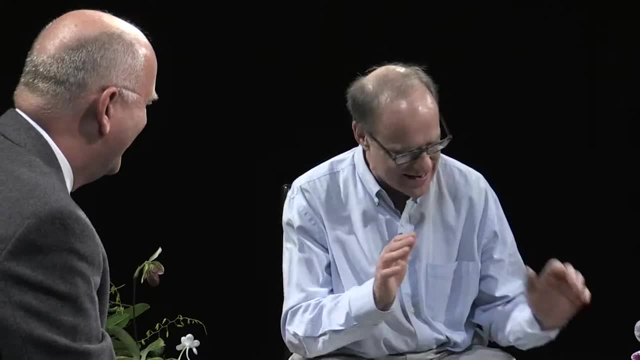 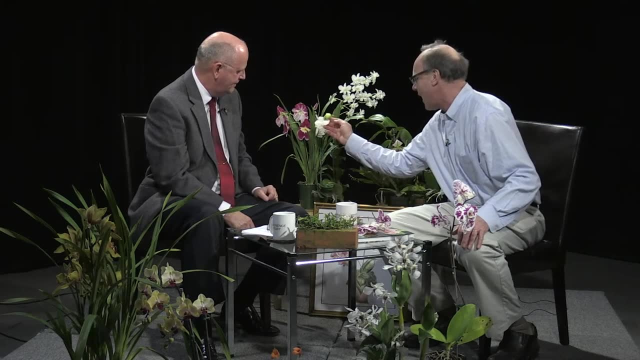 There's no way we can get you. you know, if you can just come out here with learning one name. they all look alike. It's like this one here. they all have these same little leaves that come down and they're flat, and they also have these little white. 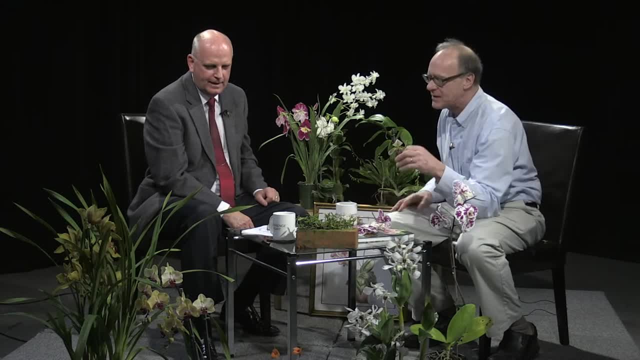 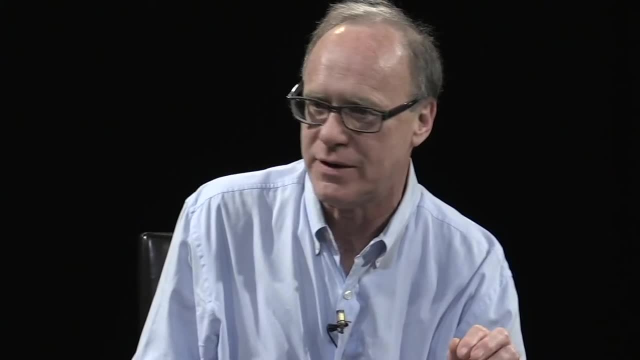 yellow, red flowers like this one up there on the top. so there's little leaves of that. That's pretty much the standard of America. These are produced by the millions and millions, and Taiwan is one of the chief places that produces them. 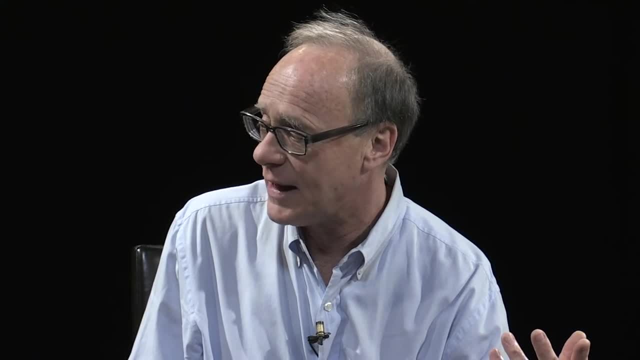 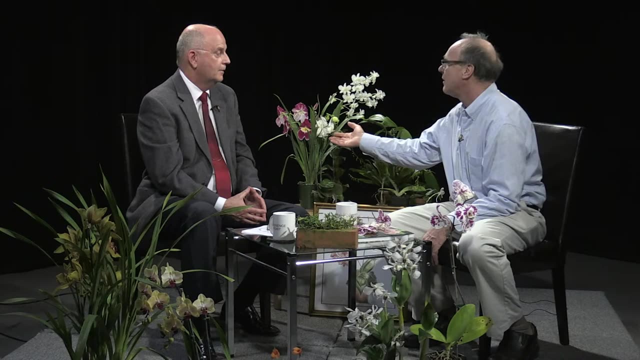 and we import them here. And this is all pretty new technology. 30 years ago, this common Phalaenopsis which you can buy at Trader Joe's today would have been like $75 at Trader Joe's if you could find it. 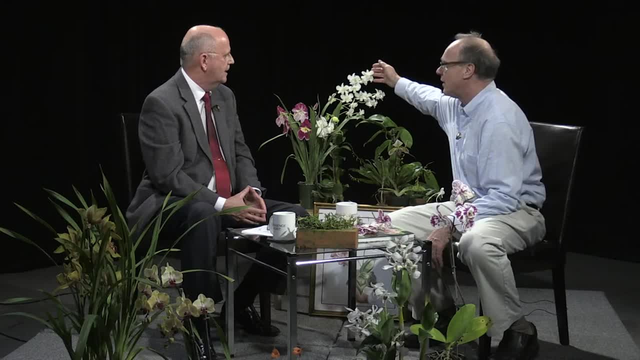 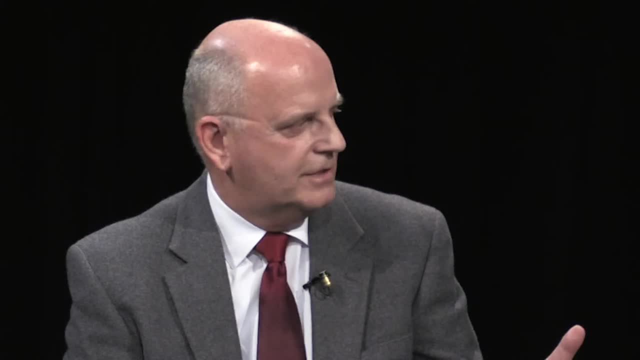 And at that point this Dendrobium was actually a more common orchid. 30 years ago, This is the one they started producing in Hawaii and also in Malaysia. I wanna touch on something because you mentioned Taiwan and you mentioned Hawaii. 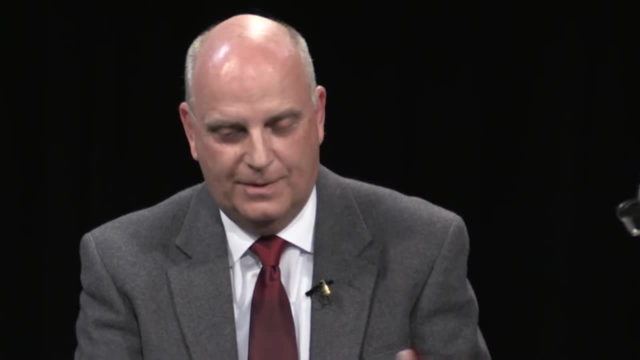 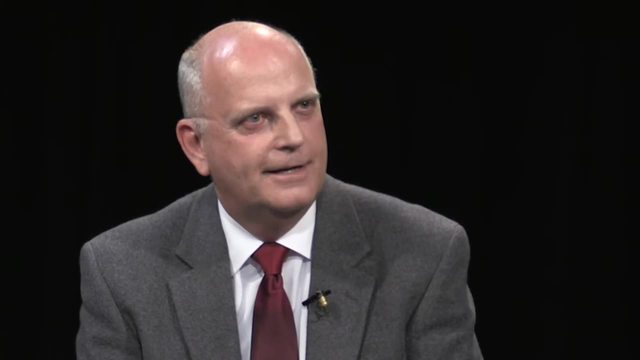 and you kind of, I don't know, for some reason, when you think orchid, you kind of think tropical- Yes, you do. But is that? but that's not accurate, is it Not at all? They have, we have orchids right here in California. 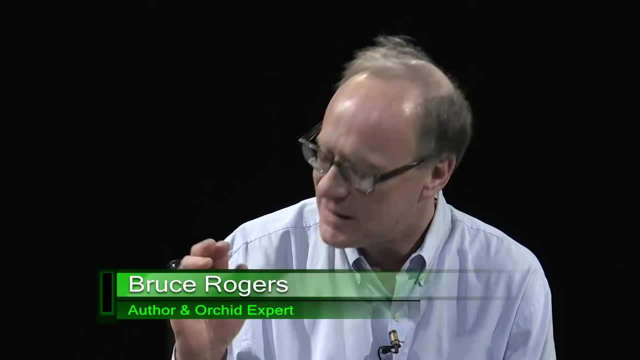 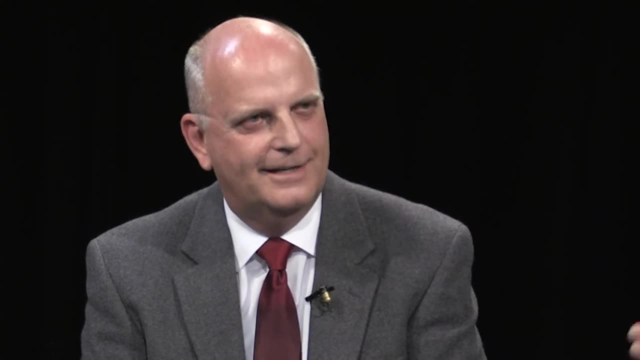 We have orchids right here in this valley- we're in here- That are native to this Exactly. There's a lovely little one called Calypso balbosa that grows underneath all the redwood trees. So Michigan, the redwood trees, Muir Woods. 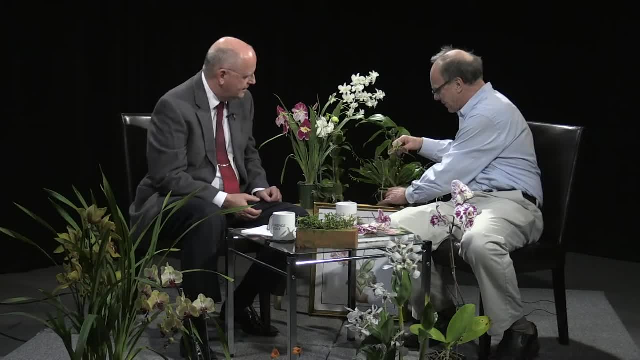 the Santa Cruz Mountains. It's a little lady slipper. It's much like this lady slipper. here, The lady slipper is an orchid. Yes, this is lady slipper as well, Only the Calypso balbosa, our native orchid, is this. 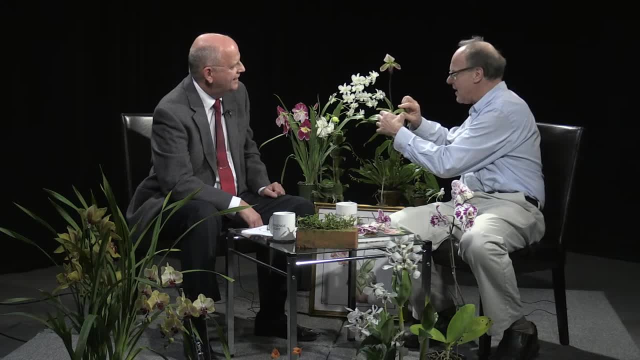 but it's only this tall, Oh nice, There's like a miniature one of these, and they hide underneath the and great history with medicinal use by the local native peoples as well. Well, my family and I, my wife and kids and I. 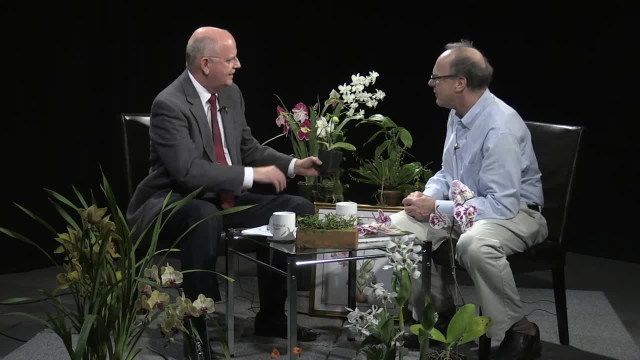 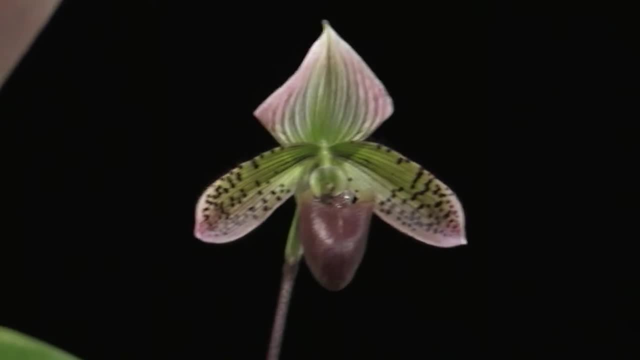 lived in New Hampshire for a number of years. That's nice there And these ladies we'd see out in the back on our 12 acres, these things, these lady slippers, they would pop up and they would and, for whatever reason, I never considered them. I never knew they were an orchid. They're one of America's best known and best loved orchids. Actually, with these lady slippers, they all call them lady slipper orchids. When they occur in Asia, they're called Paphiopedilum. 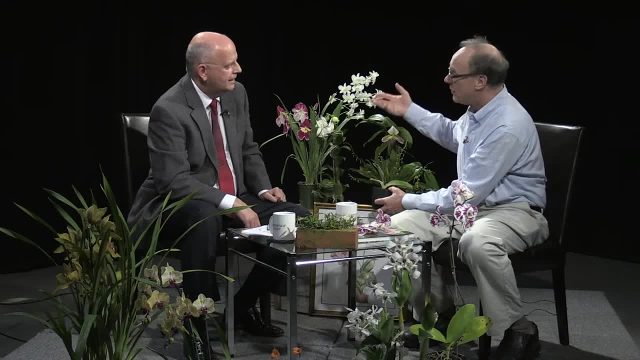 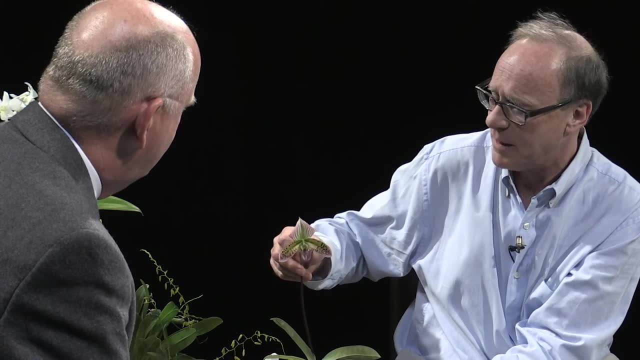 When they occur in South America they're called Phragmopedilum, When they occur in America, Cypriopedilum, And so. but subsequently they're all just basic lady slipper orchids. They all have the same little pouch that they have. 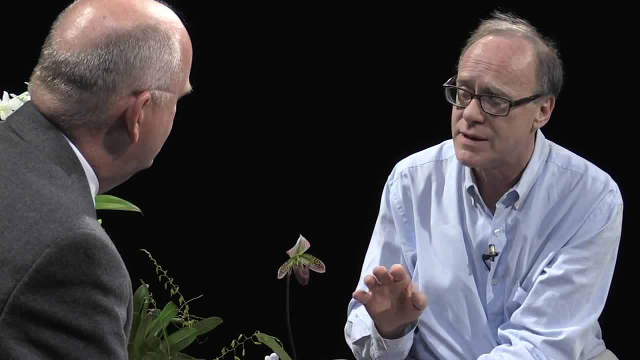 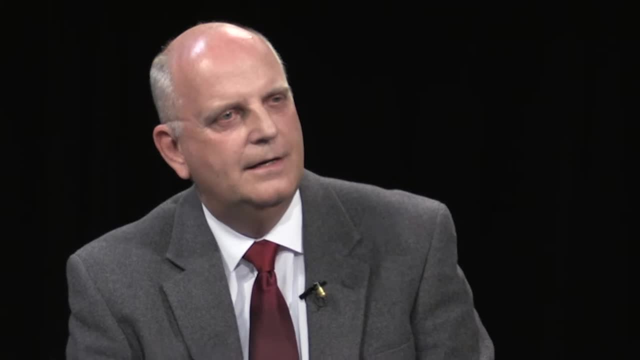 How cool is that? And actually it's very difficult to grow our native orchids in cultivation. The only place you can do that is basically back east, where they're growing in the ground already, If you take those orchids from back east and bring them to a greenhouse. 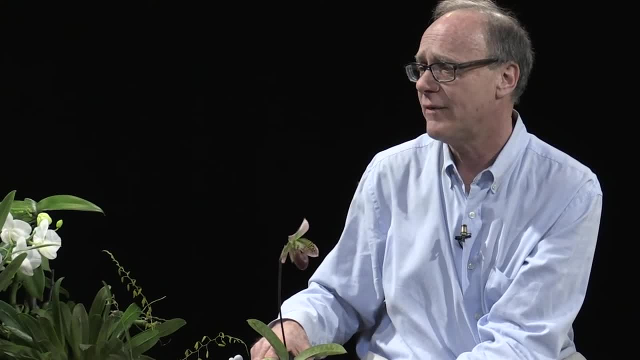 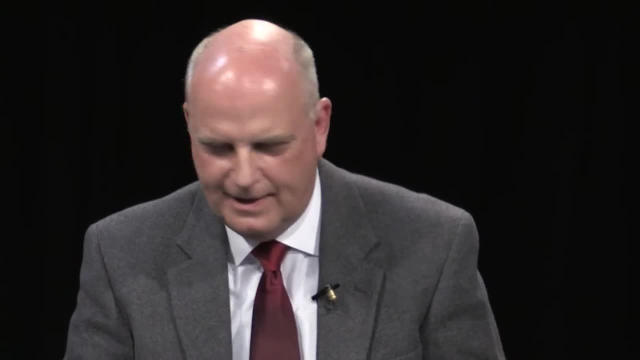 it's very hard to duplicate good culture in a greenhouse. for a native California or a native American, The American orchids, the ones from back east, for example. So if I'm, you know, here, I am Dave and I take- oh, this is really, this is beautiful. 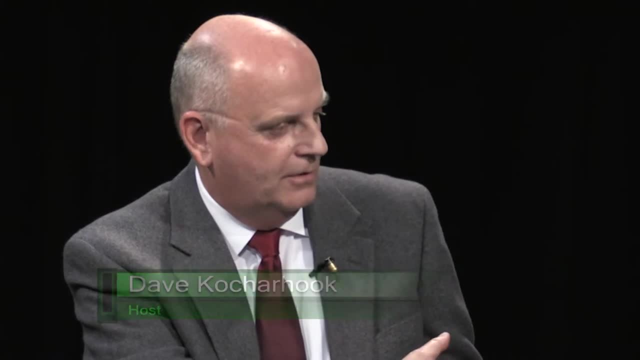 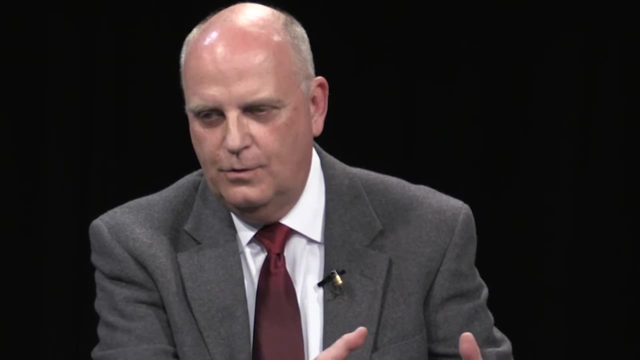 This orchid is gorgeous or that orchid is beautiful. I want to try some of these, or grow some of these, or at least have some of these in my house and stuff like that. You brought these samples, but you're a specialist. 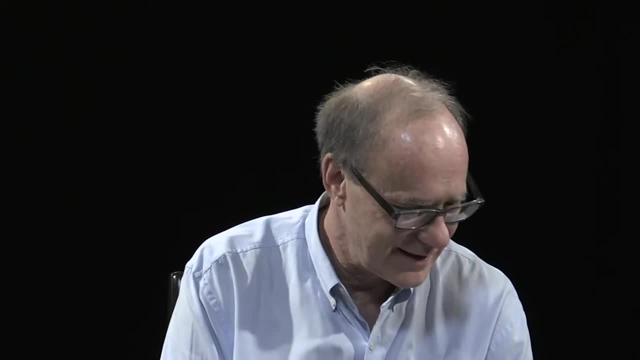 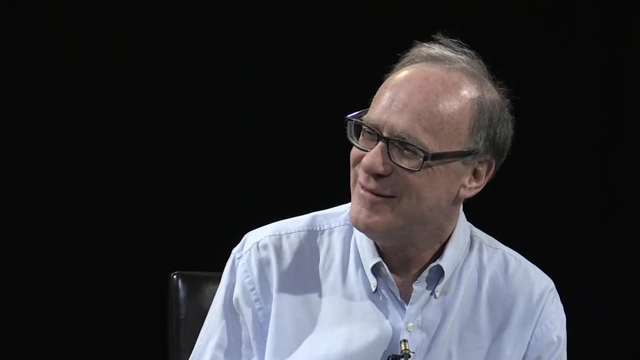 You know this stuff. Yes, we do that, This one that you mentioned. I kind of get how we can keep that one going, but what do you do for some of these other beautiful things? We've got to give you an easy one, Dave. 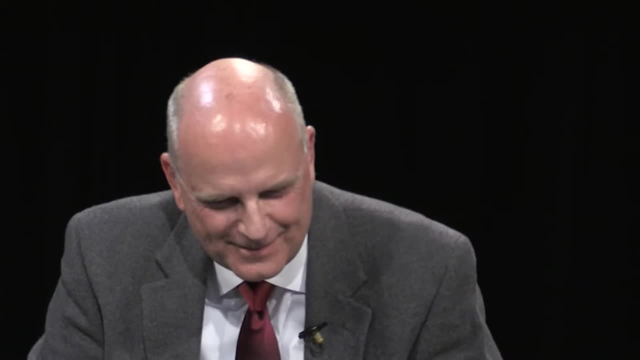 We've got to give you some easy ones. I need something easy, Otherwise you know you're never going to buy them anymore if they don't start blooming back. If you look right in front of you, this taller gold one right here. 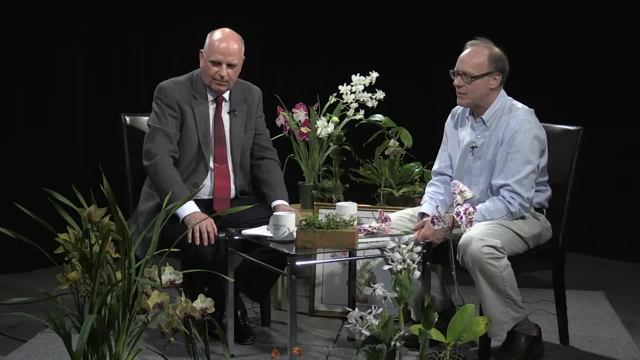 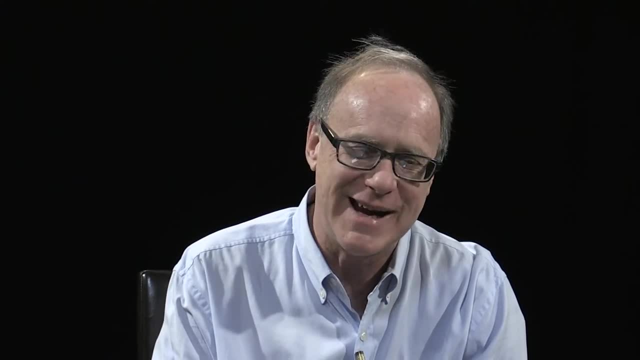 that's called a Cymbidium. That is one of the most common orchids we have in North America. a big history in this And this is a North American orchid. It's native to North America. No, it's not. 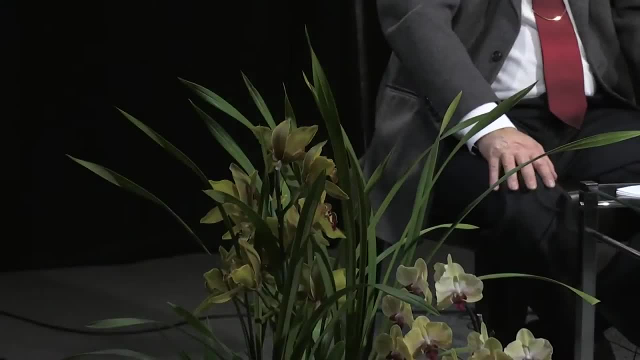 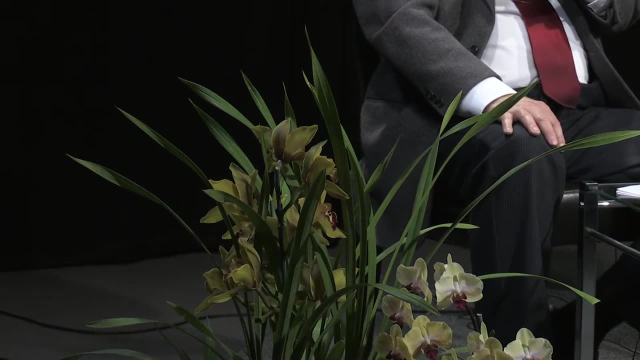 It's native to Asia, Native to Asia, But it'll grow outside in North America, Okay, okay, Because it's from regions in Asia that are similar in climate to our climate here, Which I was interested in because you mentioned that this one, the Lace Slipper. if you take it out of its stent, normal environment, it has a challenge growing elsewhere. Absolutely, Cymbidiums. they grow right outside in Santa Fe. They're very hardy, Very, very hardy, And not only do they grow outside here. 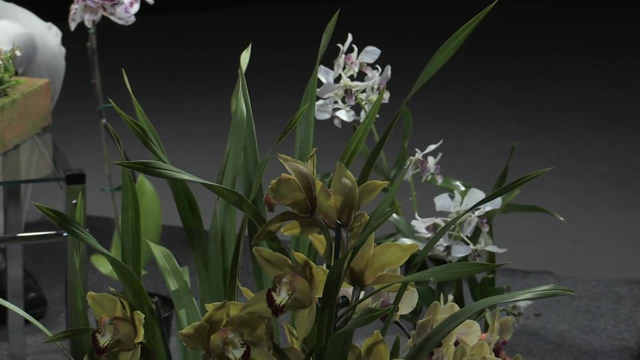 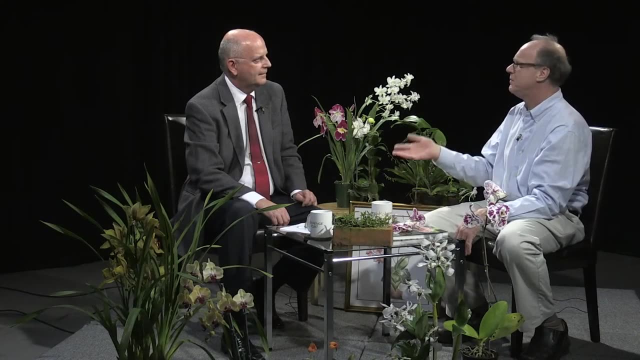 but they thrive out here And there's a local, a huge history. We used to have a firm called Rod McClellan's And for a while there was a whole. it was a big deal every Mother's Day. There were literally hundreds of thousands of Cymbidiums. 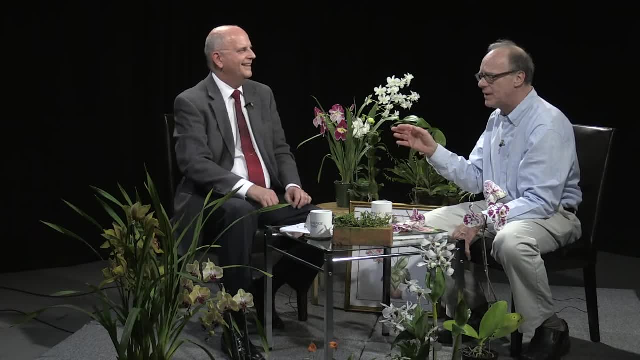 I worked there. that's why I know that They would be produced for Mother's Day and stuff A big deal. Now what's happened with these Cymbidiums? you might notice that nowadays they've gotten shorter And the flowers have gotten a little smaller. 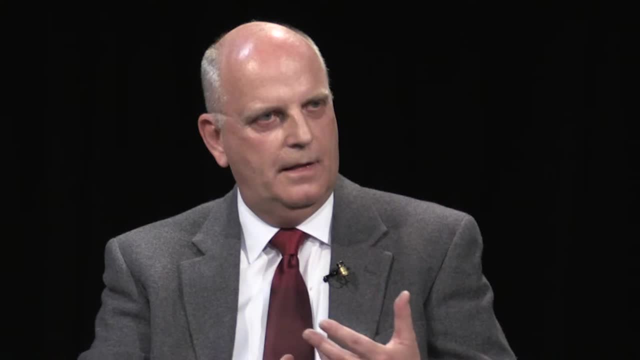 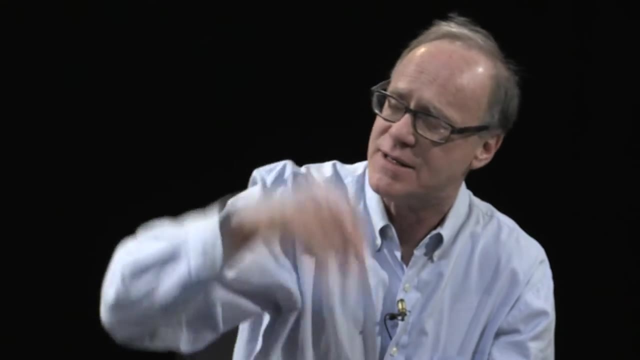 to make them easier to ship. Oh, so they. that was a planned, Exactly a planned- attack to reduce the size of these Cymbidium orchids, Because before the plant would be twice its size And shipping was a nightmare. 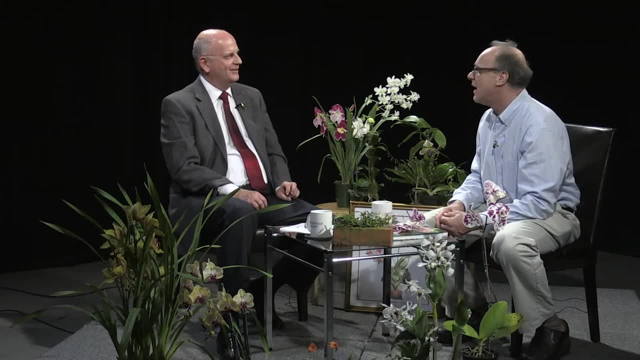 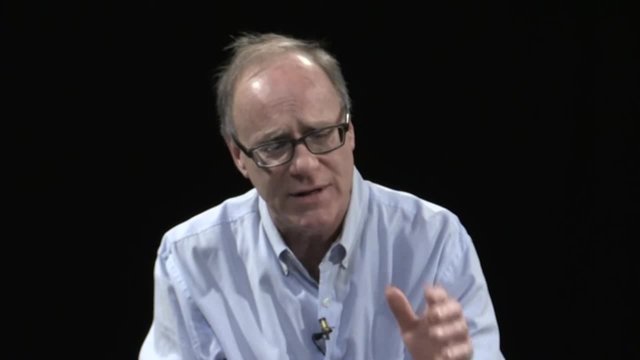 Yeah. So subsequently one of our local Genetic engineering, so to speak, Mostly breeding just down, straight breeding, And as it was brought, they reduced that to a smaller size And that one does very, very well outside, Also multi-colors. 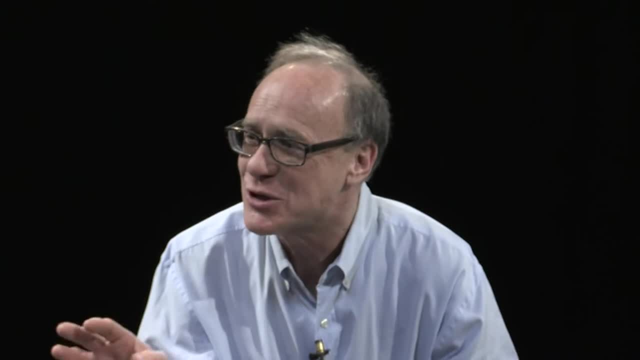 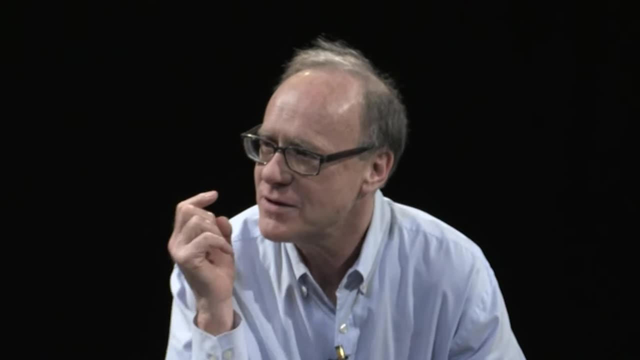 All colors, from whites to pinks, And also the best when you're shopping for orchids, Dave. Next time you go shopping, and even if you're Best Buy or whatever, I want you to incorporate your nose, Because the first thing that falls down genetically. with orchids is scent, And with scent you have the whole shebang. Yeah, You get the flower, you get the scent, But the first thing that falls genetically is scent. But if you look at that Cymbidium there, it might have a slight fragrance in the morning, but if you go out Cymbidium hunting, when you go out to your store to look at Cymbidiums, I want you to go around there and sniff each one of them. 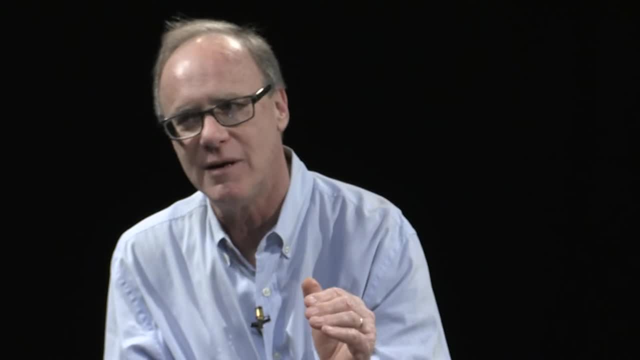 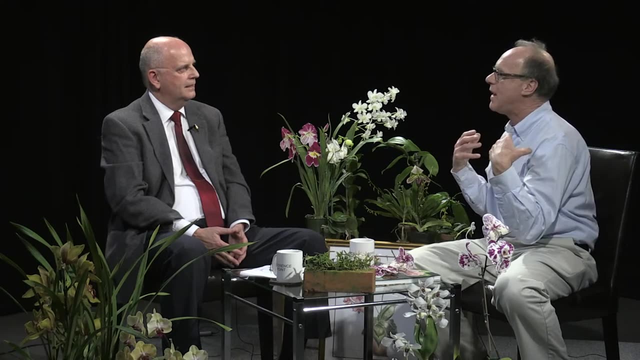 Because there's some, because now people are starting to breed for fragrance again. People, the breeders, realize: well, this is a lost opportunity here. Everybody loves the whole package, Everybody loves fragrance. So incorporating breeding back into the Cymbidiums. 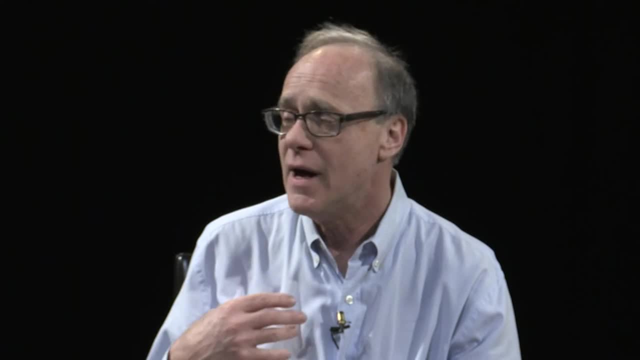 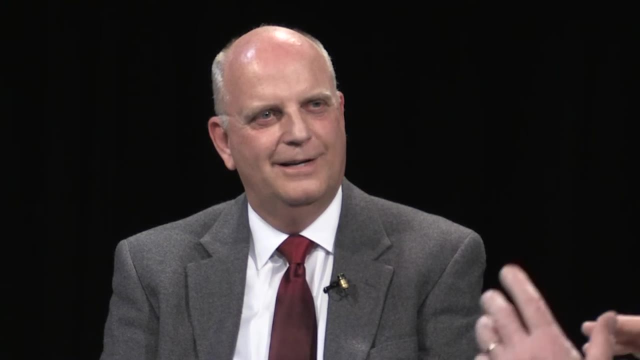 Interesting, And I breed an orchid myself. I breed an orchid called Sebrella And we actually breed just four fragrances with that plant, Fascinating. We have a specific lemon-lime scent or something. Oh, how cool. 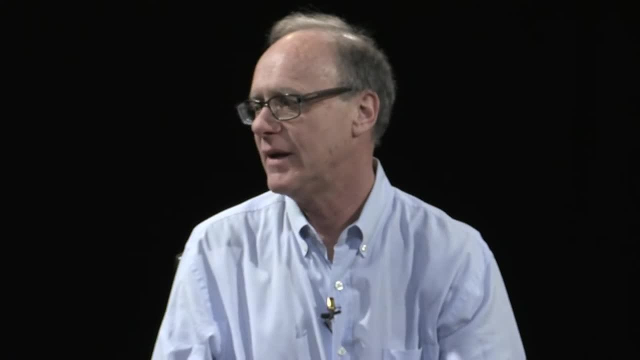 We don't care much what the flower looks like. We're going for that scent Nice, Because it kind of makes the whole package, Because that's one of the things that's been lost over the years- is the-. Well, yeah, I noticed. 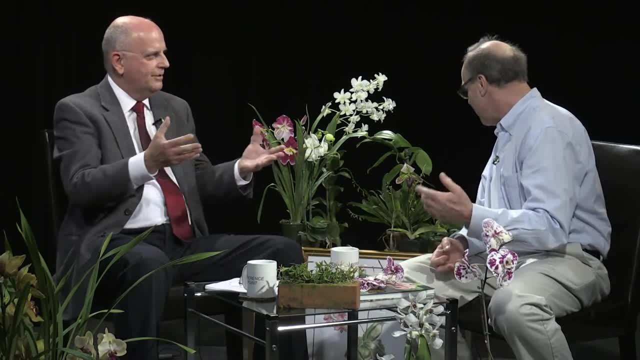 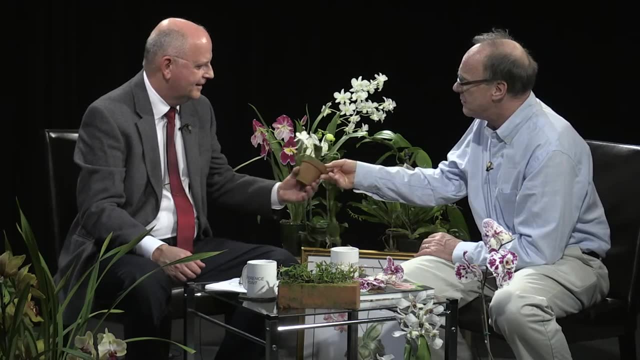 So we're sitting here amongst these, and if there were a bunch of roses or something here- We'd smell it. yeah, Very few are fragrant here. This is one that might be a little fragrant right now. This is a little miniature Angraecoid from Africa. 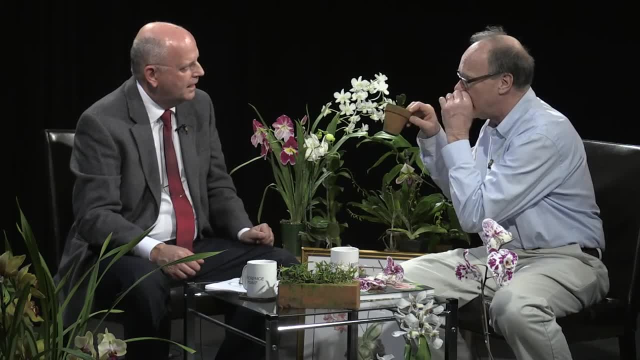 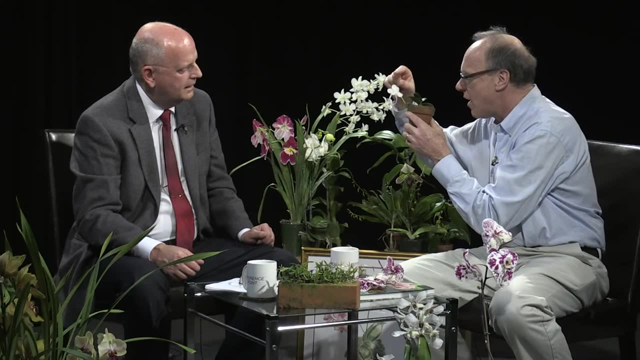 You can smell it. That's because it's pollinated by a moth. This is like Darwin's orchid. It's like a miniature replication of Darwin's orchid. Can you see the nectary here? So the moth, the moth that pollinates this- has a tongue long enough. 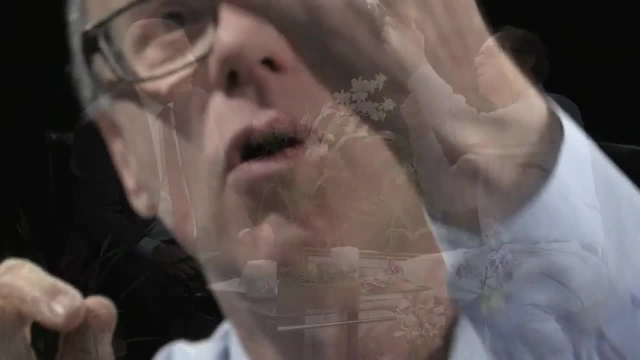 to get to the nectar at the very bottom of this nectary. Oh, how cool is that. If you hold it up to the light, you'll see there's a little bit of fluid in the very end of it And that's what the moth is going after. 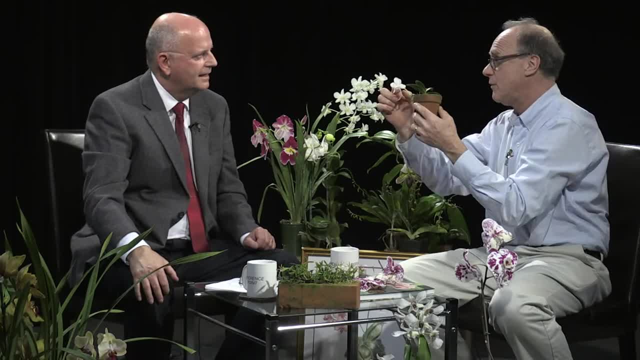 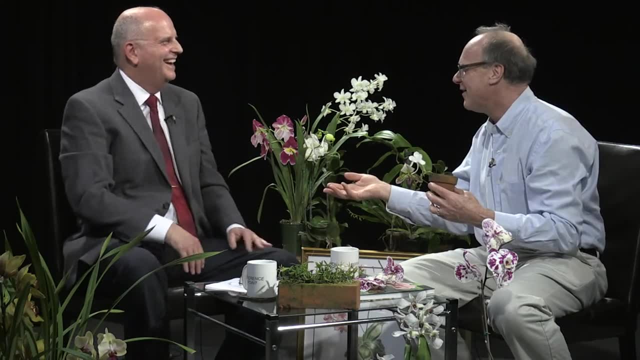 And that's what Darwin said when he found a flower just like this, but the nectary was 14 inches long, Wow. And then, 10 years after they died- isn't that just like life. They found the moth. He must have been mad about that. 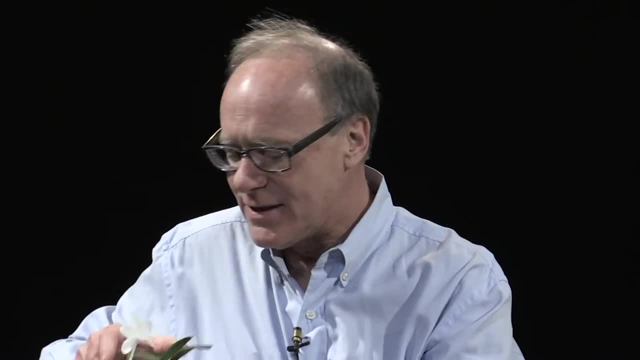 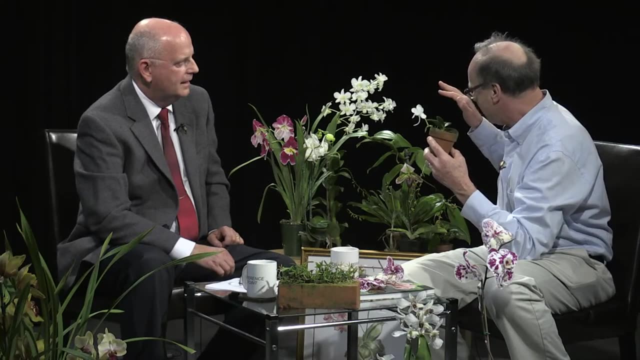 I told you guys that moth was here, It had to be there somewhere, It had to be there someplace. And this is like a little warm-growing orchid. Now, when you have them growing orchids in your home, you see there's large ones and there's small ones. 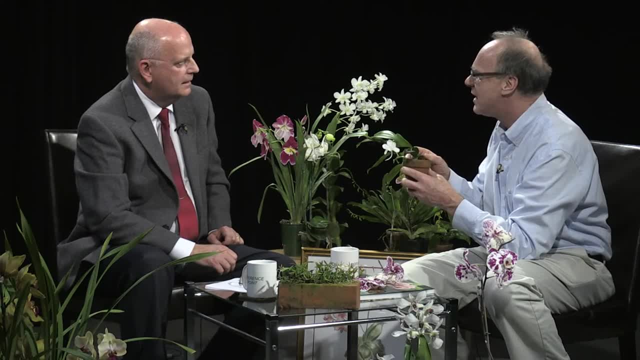 medium-sized ones. This is one of the ones that stays a small orchid And it stays warm and it grows warm. This could be grown in the house with your Phalaenopsis. That's the biggest thing. So, having it indoors or outdoors- 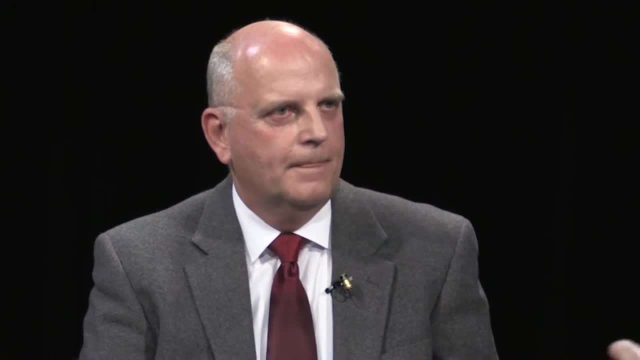 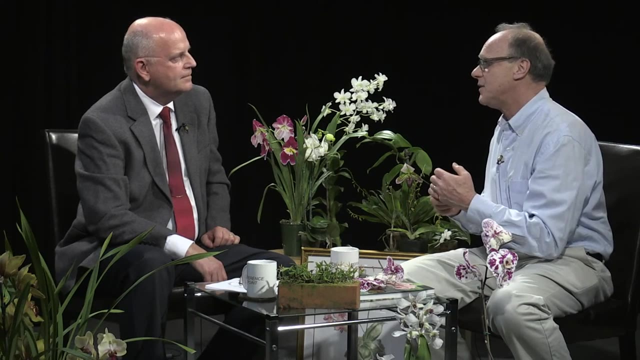 depending upon the Exactly. That's the best thing. So whenever you buy an orchid, whenever you're viewing public buys an orchid, they should always ask what's the name of this orchid And is it warm-growing or cool-growing? 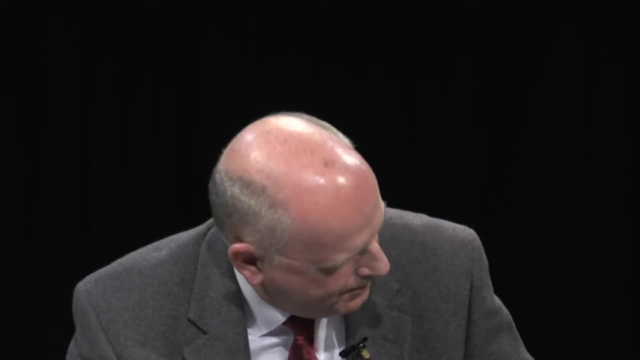 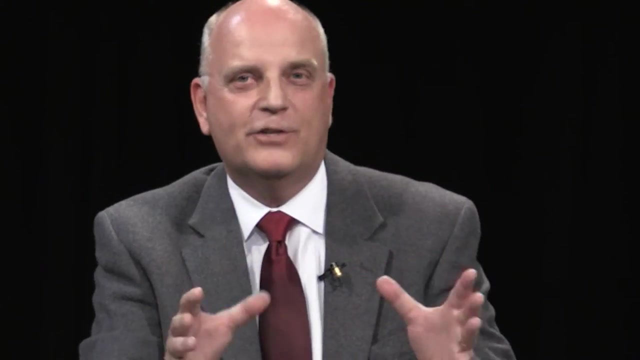 Got it And get some feedback with that. I want to talk about this plant in the back, this one right here in a moment, But as you're grabbing that, I want the folks to know that- what they can do if they have any questions about anything we're talking about. 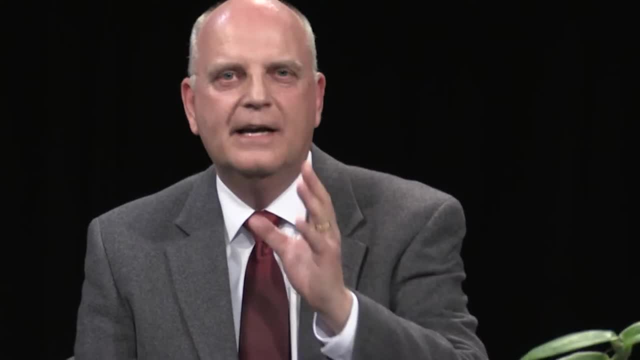 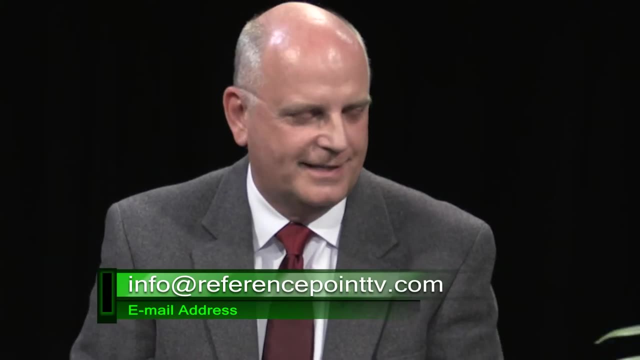 orchids or how-tos or recognizing things. send us a query. You can send us an email at info at referencepointtvcom. I'll get it to Bruce, He'll answer your questions and we'll get that taken care of. So what we have here is what. 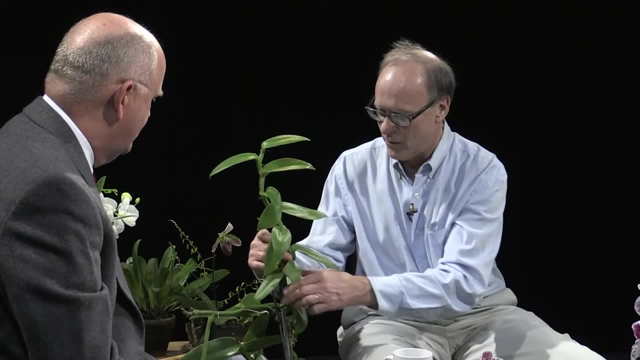 The famous vanilla orchid. The vanilla orchid. This is the vanilla orchid. If you were a tree, This is what vanilla beans come from. This is what vanilla beans come from. What happens is, if you imagine, we have to imagine this. 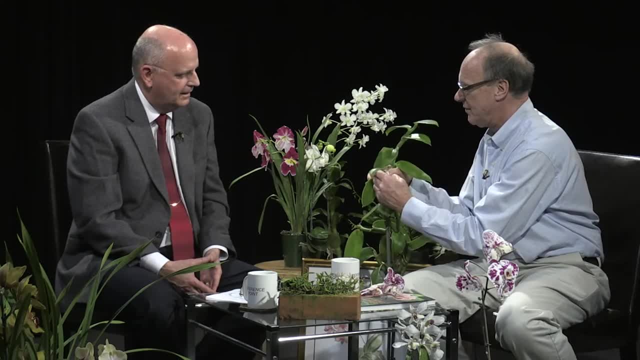 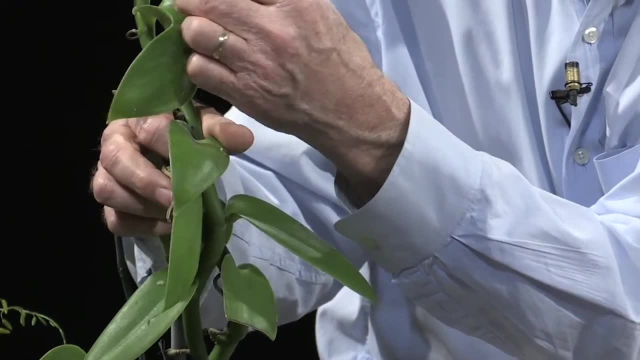 Pretend this is like an all-white flower. It's about this size too, So I'm going to just crumple this down to make it look like a little teeny all-white flower, Which you'll see. this produces one flower right at the axis of the leaf node. 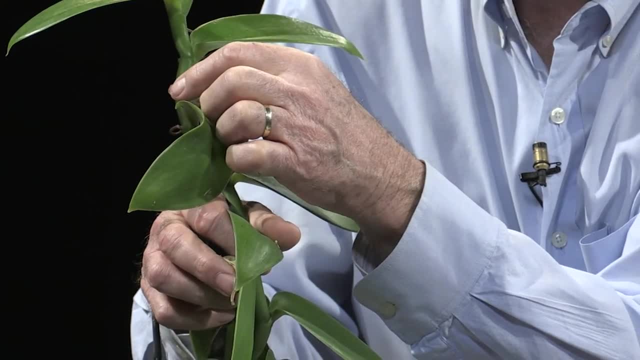 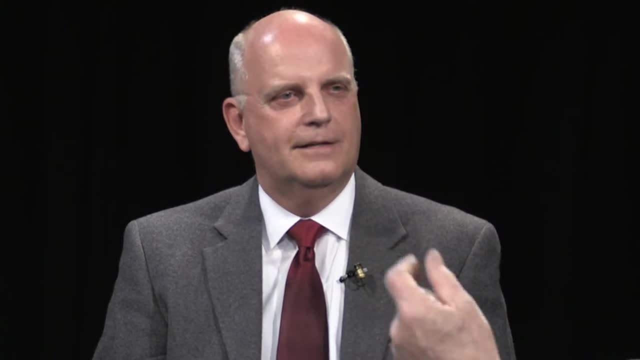 And this one flower is pollinated by hand. Then it forms a seed pod. Yes, And the seed pod is like a long bean, And that is your vanilla bean, And that is where vanilla comes from. How interesting. And this is probably the most. 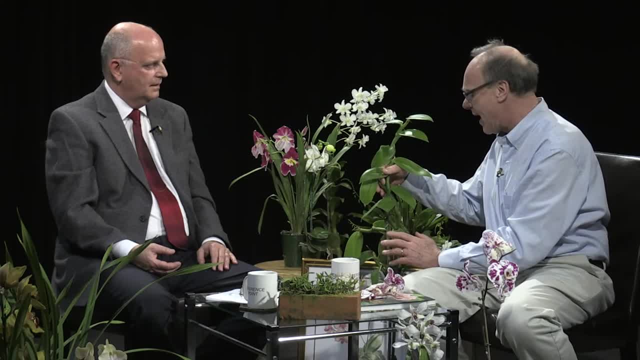 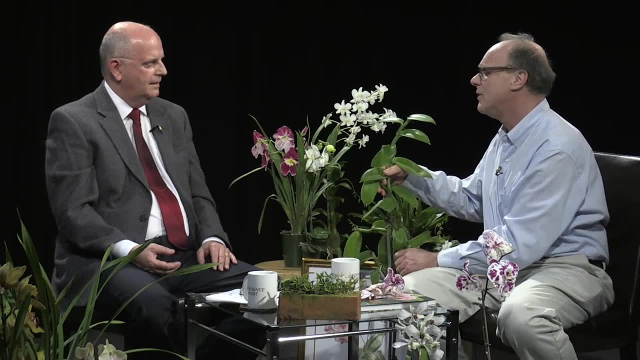 People used to think this was the only orchid people use for food, and what have you? But the reality is people have been eating orchids all around the world forever. Wow, That's one of these misconceptions that we have is that only this orchid is used for food. 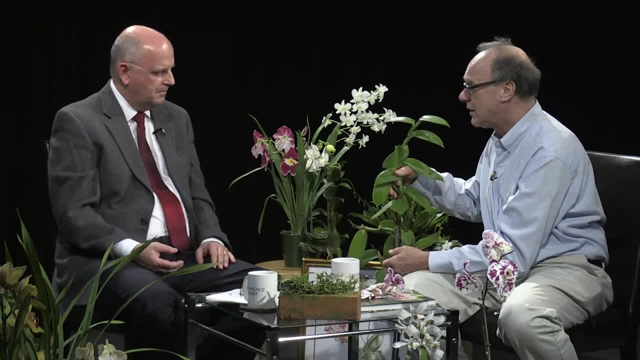 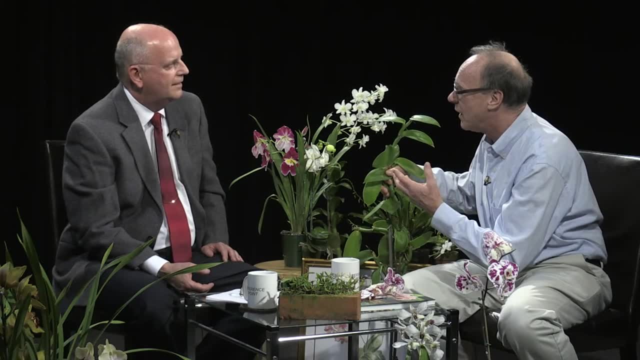 But in reality there's a whole bunch of terrestrial orchids that come like, for example. Africa is having a huge problem right now because they make a meatless bologna out of orchids in Africa And it's gotten so popular in Zimbabwe. 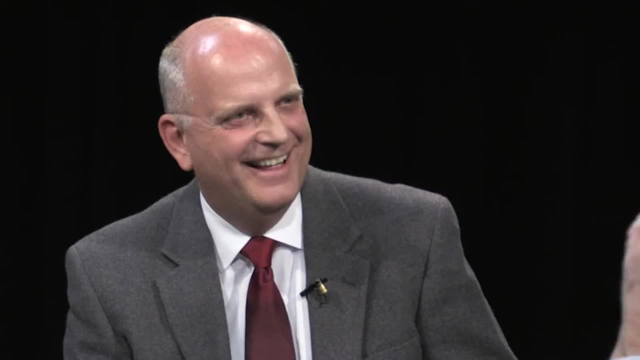 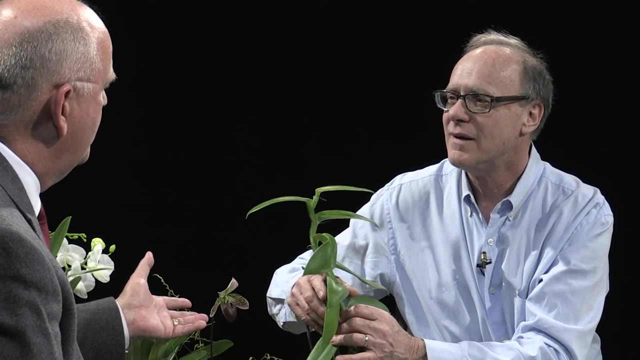 it's completely extinct? Oh no, And so now they are smuggling tons of these orchids across the borders From other countries. Oh my goodness, Just to keep up with this. Could they cultivate them if they wanted to? It's very difficult because they're native orchids. 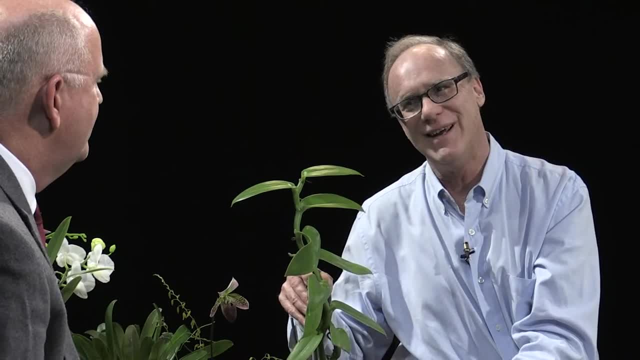 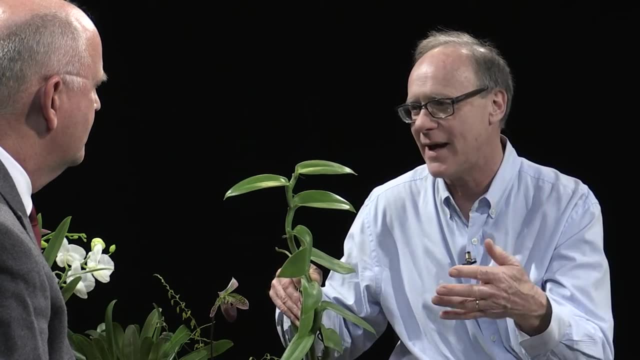 just like we had talked about, Ah yes, The most difficult kinds of orchids to cultivate, Nice, And so subsequently they're like the whole thing with the orchids. they've called me to ask for what do I suggest? because in their native habitat, 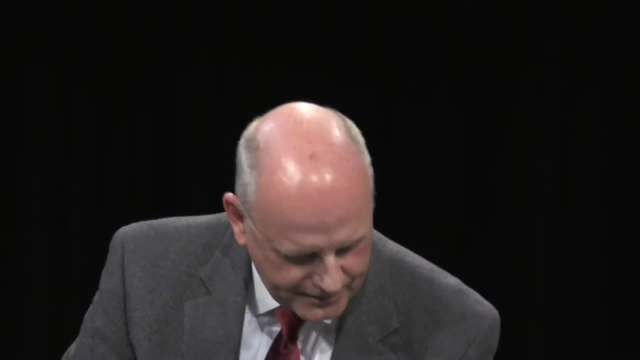 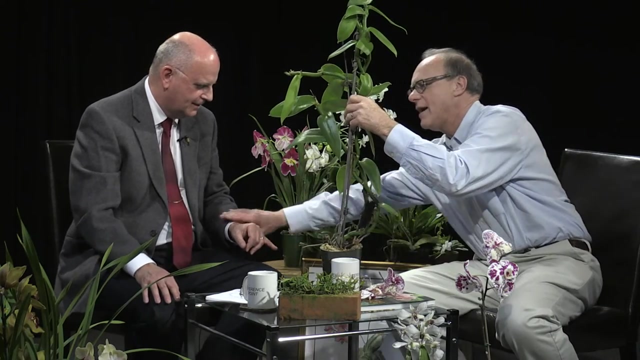 they're now extinct or approaching extinction- Interesting. Okay, could you lift that up for just a moment? Sure, of course. I want to point something out and ask you about this, because it looks like these roots, These are roots Now, David I. 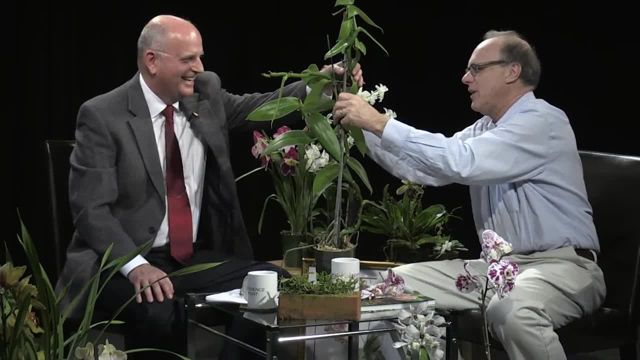 You got to pretend like you're a tree. You're a tree, All right, I'm a tree. Okay, you're a tree, I'm a tree. Now what this root will do, like, for example, this little root here: 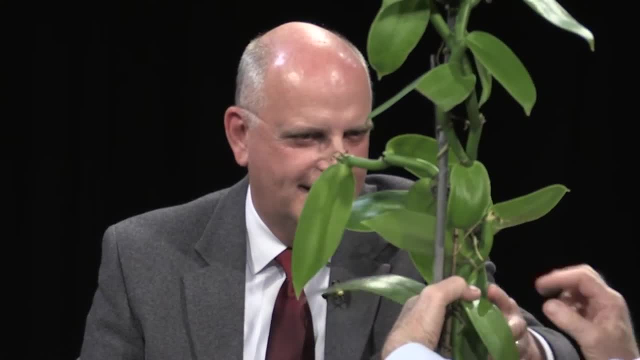 let's bring you down right here. You're a little tree and you have a little branch here. This root here will wrap around your finger. Maybe the camera can see this. Maybe the camera can't see this. Okay, yeah, yeah. 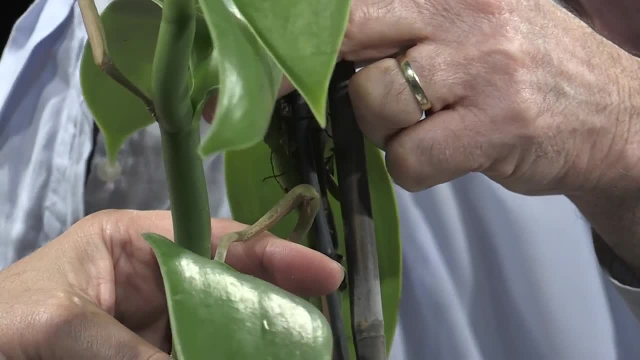 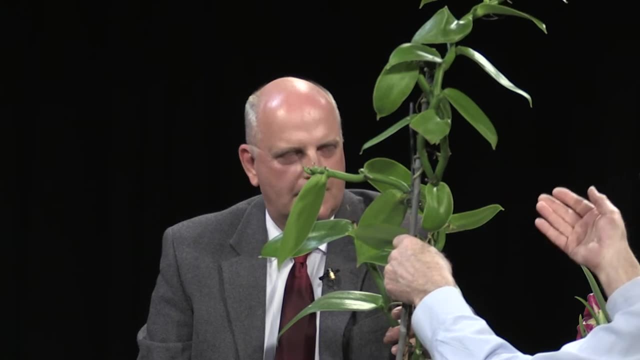 And it hatches itself to the tree, And so it grows flush right on the tree, And they grow them in the shade of trees. Sometimes they grow them under coffee. Okay, There's a whole Mexican lore about the cacao tree. Yeah, yeah. 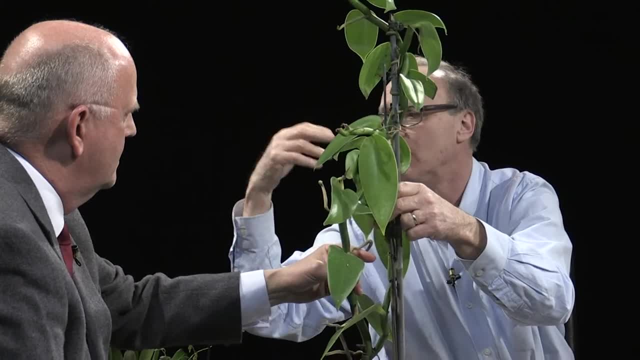 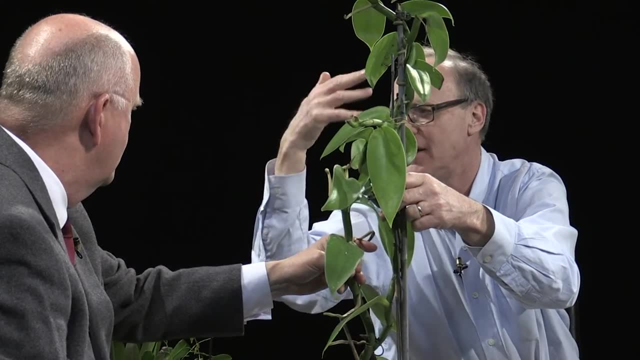 And then also the vanilla growing together. There's actually a myth that the vanilla was one Mayan princess and the cacao was a Mayan prince And they grouped around. They had a lot of fun in Orchid Paradise And they got, but they were too naughty. 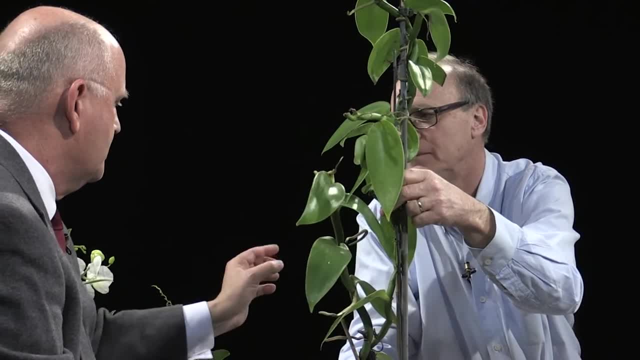 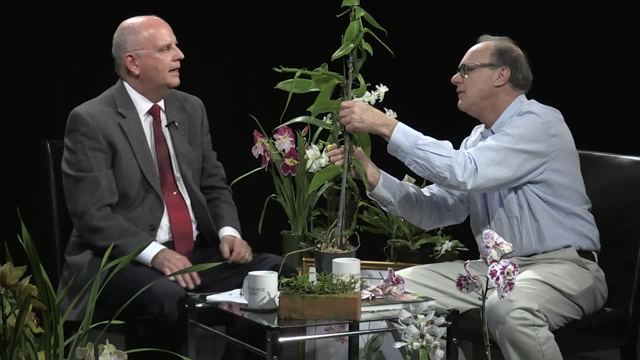 They were too naughty and they were changed into plants. But not all orchids have this root-like thing. No, this is probably one of the very few that actually even grows like a vine. That's very, but there's so many different kinds. 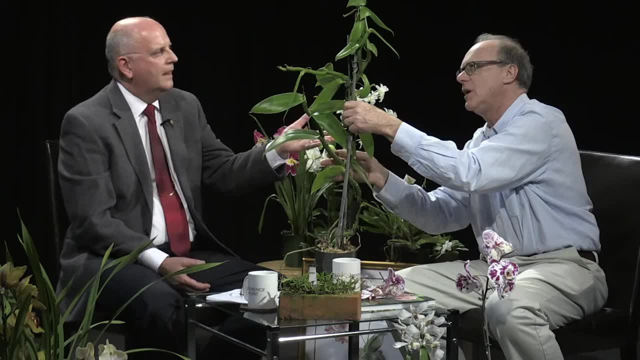 of orchid. David, That's what's gonna be so exciting for you. When you go to the orchid show, you'll see all these plants. Let's talk about that. Tell us about the show coming up. Oh, it's exciting. 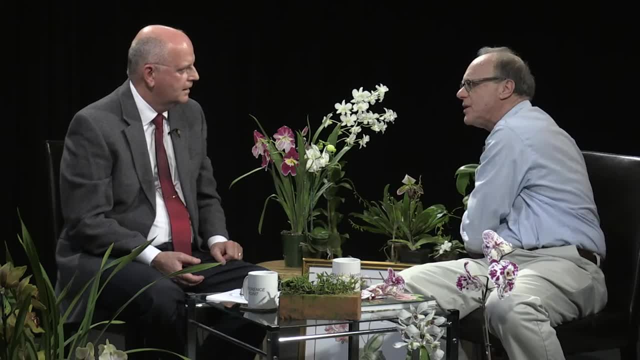 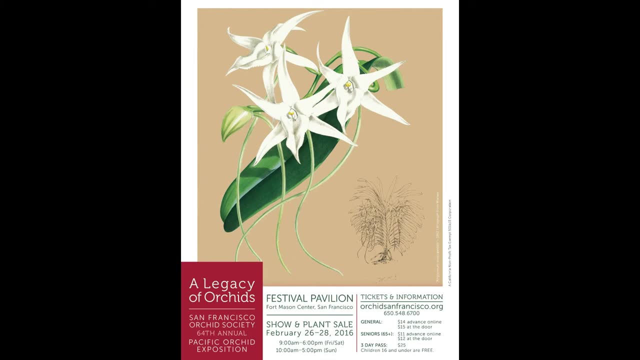 It's a very Historically it's one of the most important shows in America. We have a huge contention of orchid growers here in California, Very, very well known, And we're able to do more with orchids in California than, let's say, they do in Florida. 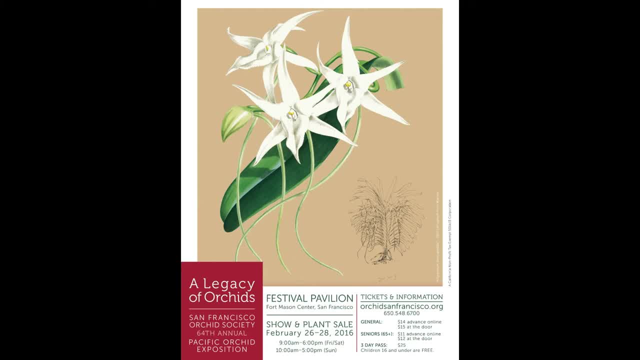 Why is that? Because of our climate. Because of our climate, See, we can grow warm things in our warm greenhouse And orchids that are cool growing. they actually need to be. Hand me that one and I'll set that up over here. 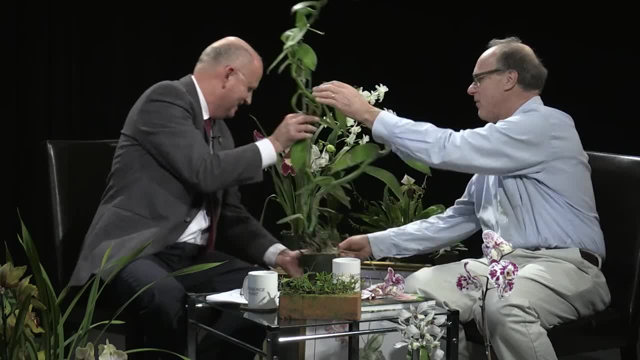 so you've got hands free. Face this, get this guy over here. Watch out, it'll just attach right to your leg. There we go, it will never leave. And actually what they do in homes. I've seen them attach. people grow them on their kitchen windows, on their eaves, and the roots attach so solidly to the wood that when they peel off, it peels off all their paint. I've seen that, Yeah, so it's very easy to do. 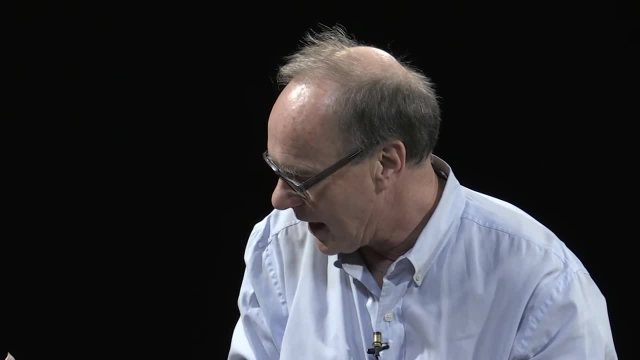 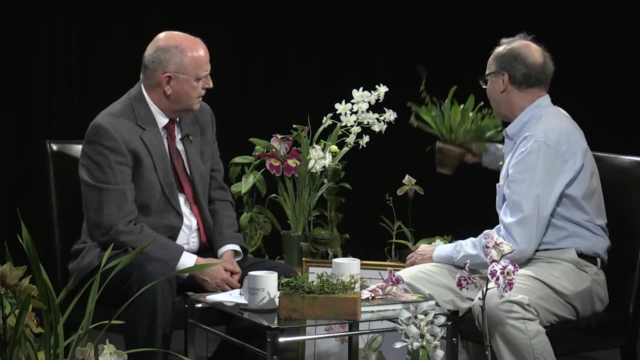 So we have some cool growing orchids And there's, for example, on this table here I mentioned, this little small one is a worm growing orchid. But here, for example, just to show you how odd and different these are, this grows right outside. 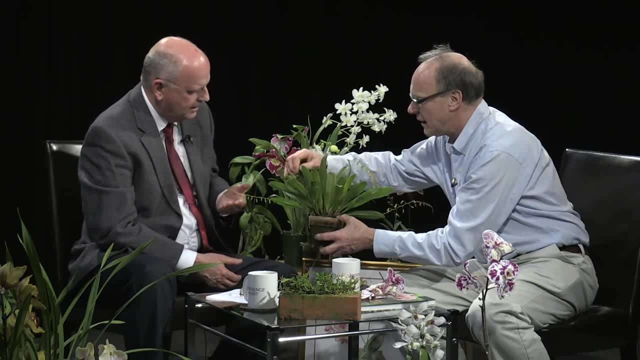 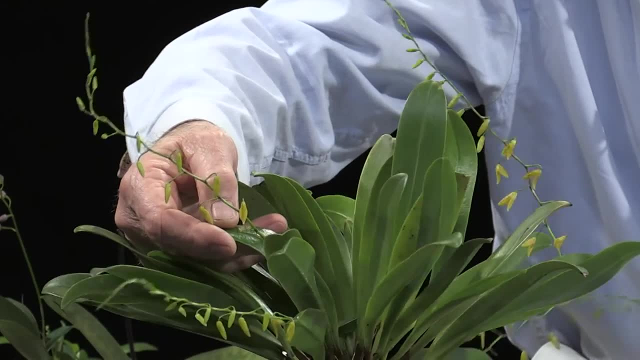 Isn't this a crazy tiny little flower. But look, what's even more exciting, Dave- Maybe we can show the camera at this- is if you look out where the stem comes out of the leaf. It comes out of the middle of the leaf. 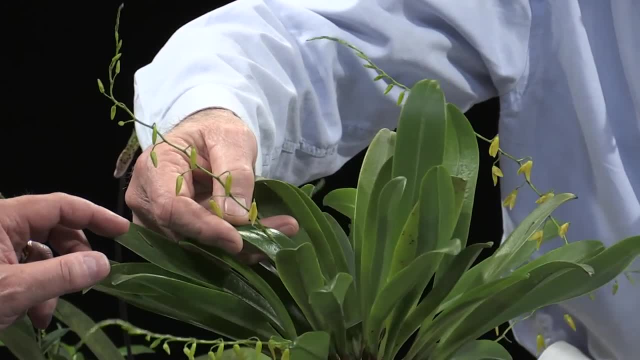 How odd is that. I've never seen something like that before. You've probably never seen any plant like that before. No, I've never seen that before. This is one of the only plants I know that even does that. I don't know why it does that. 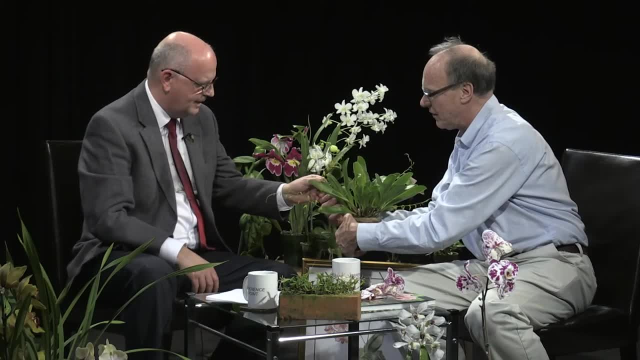 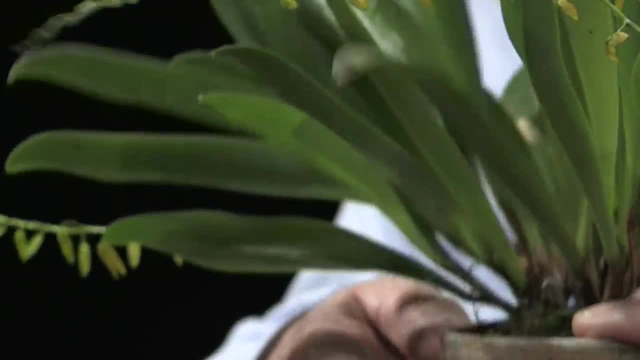 It's a good place to look at it here as well. Very, very unusual growth, very, very unusual growth And, for example, this grows in Columbia, in the high mountain, the high sea areas in Columbia, And it can grow right outside here in San Francisco. 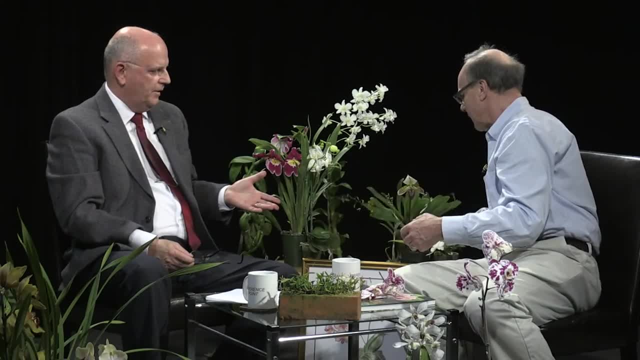 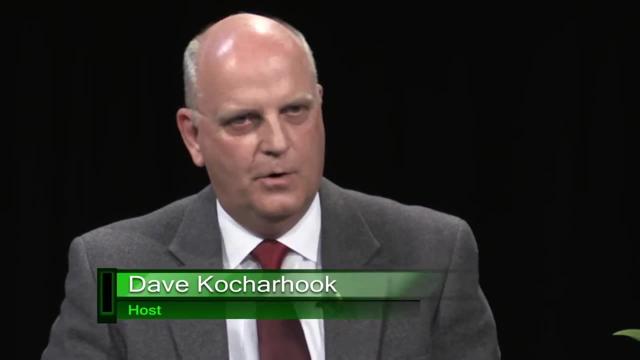 and in this area, here Let's talk a little bit about San Francisco Bay Area, because that's where we live And there are so many little microclimates here. here you know San Francisco. you come further south it gets warmer. you go on the East Bay. 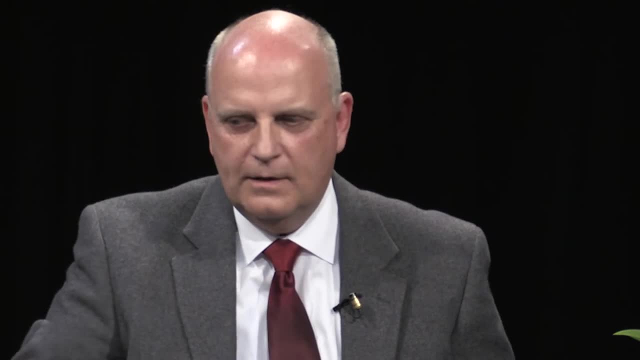 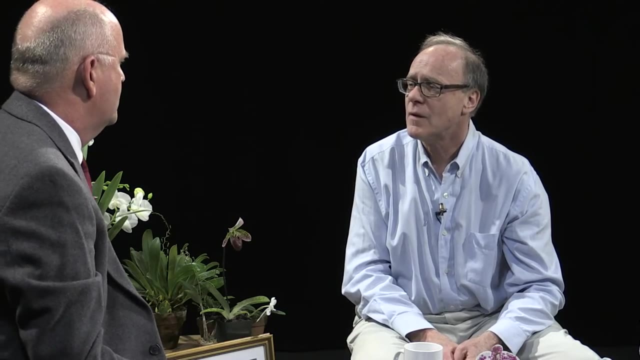 you live across in Contra Costa County or whatever. What might people want to think about in terms of the kind of orchid they might be interested in, based on where they live in the Bay Area? Well, if you mentioned before, if you have any kind of yard space at all, then you want to, of course, go right to the orchids that can grow outside, All right, okay, But if so, we talked about the Cymbidiums, and right to the left is this little Mazda Volia, this little orange orchid, right here. 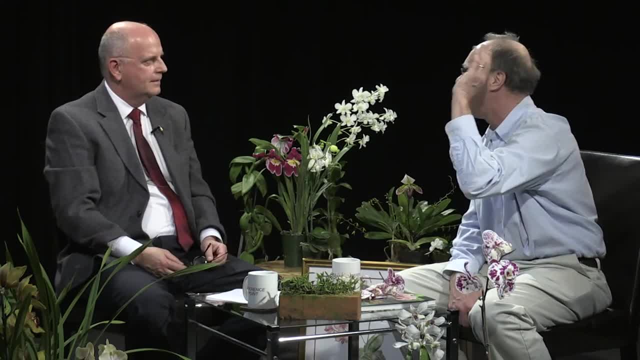 Yeah, a little orange one That grows outside so easily. You just throw them in the backyard, even down here in Santa Clara, And see in San Francisco it's not a problem at all. but instead they do well in Santa Clara too. 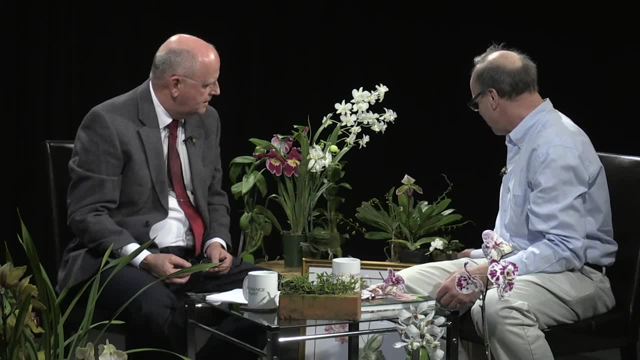 But that's about. and then this little Pleurothallus we looked at, and also this, for example: talk about miniature orchids. Look at this little miniature orchid here. Oh wow, This is another little. this one comes from Ecuador. 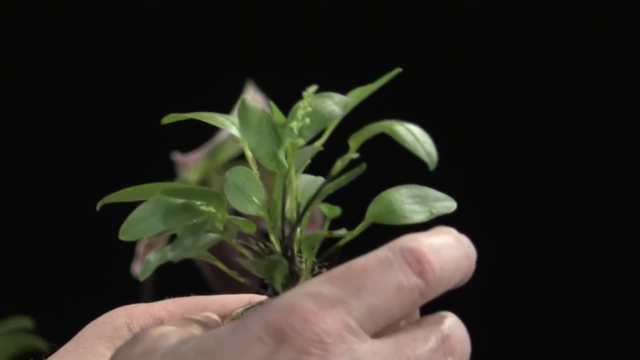 That is so tiny. Look at the little, teeny, teeny little flower. There are tens and tens of thousands, of thousands of kinds of orchids- Oh wow, More than they're finding them. still, every day We find orchid species. 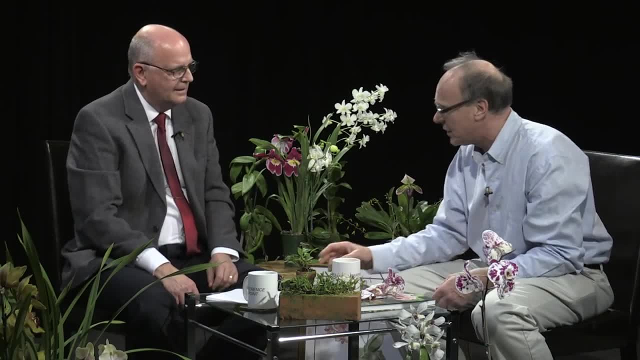 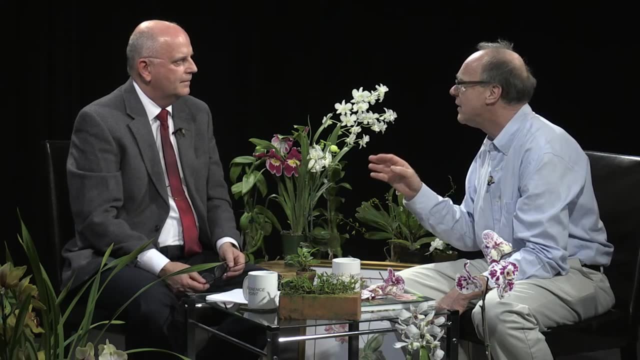 every day, and it's kind of tragic, because- from an environmental standpoint of course- because as we go ahead and we level the rain forest, we are losing things that we don't even know about yet. Let's talk about something, then. 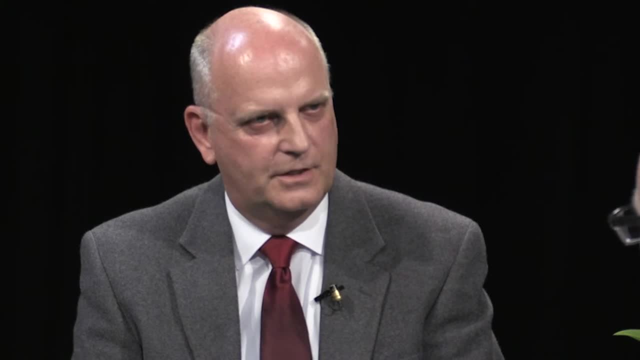 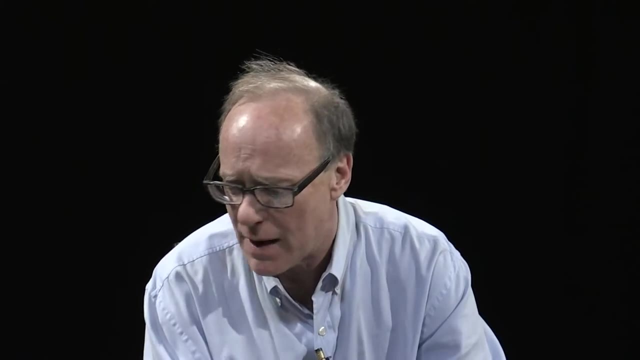 You mentioned something to me earlier about medicinal qualities of certain orchids. Yes, How does that? let's talk about that a little bit more. That's very exciting and very important. Here's a good example: This vanilla orchid we just finished talking about. 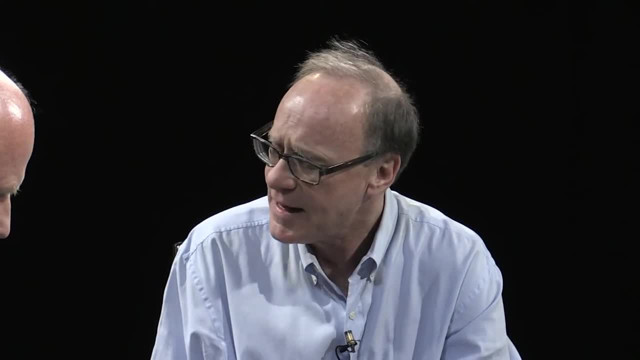 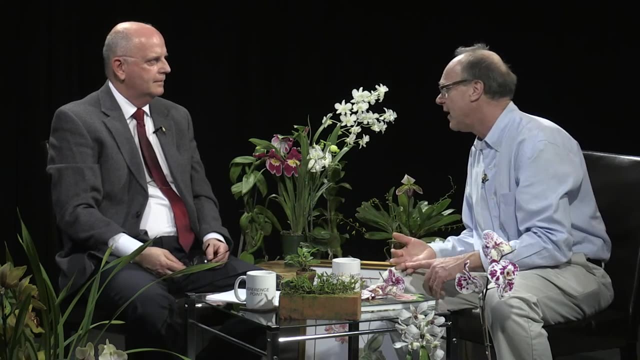 It's a minute ago. This vanilla vine is right here. This is kind of interesting. Now, how long have they been looking at vanilla? since Cortez was here, right, Right. So for hundreds of years scientists have taken it. We have artificial vanilla flavoring. 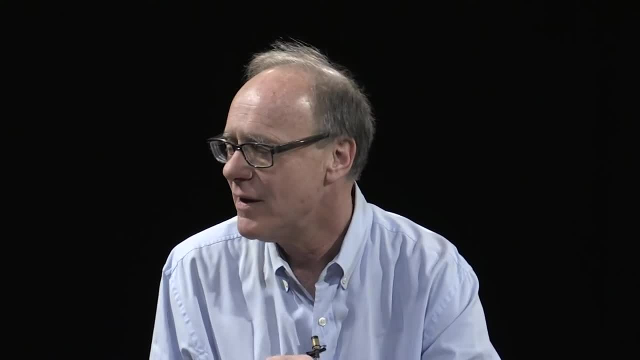 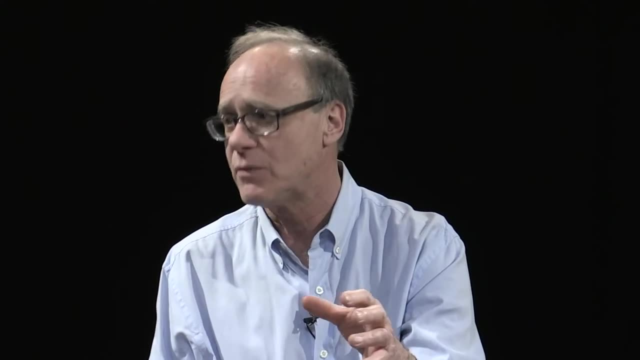 Right, We have artificial, just everything you can imagine. But they just have discovered in the last couple of years that vanilla can block quorum sensing, which is the swarm intelligence which tells bacteria when your body is weak enough to invade. Ah, You see. 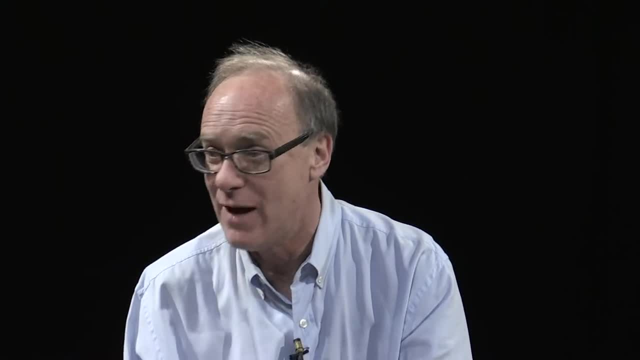 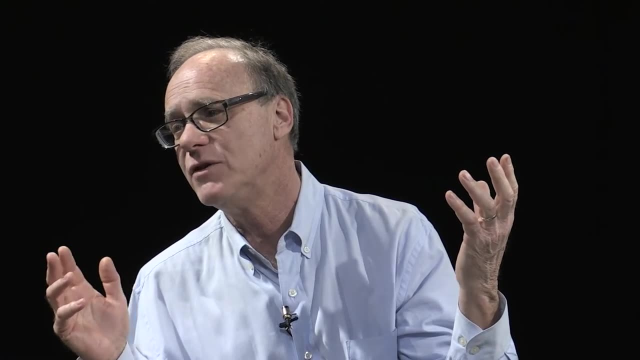 But no one knew all those years of studying vanilla and we're just now finding that out. Wow, So can you imagine the knowledge we've? we've just missed? Yeah, The knowledge we have just missed, And in terms of when I was a young hippie. 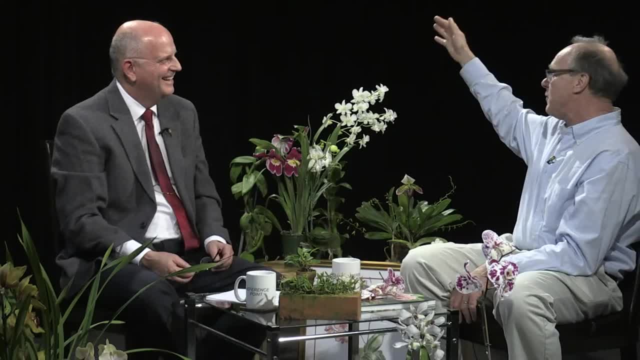 and I was growing these orchids. right, This is way back in the 60s, Right? People would say: oh Bruce, isn't there an orchid that gets you high? Can't you just smoke one of these orchids, you know? 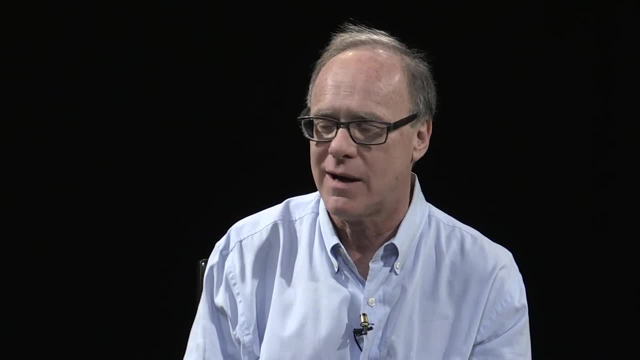 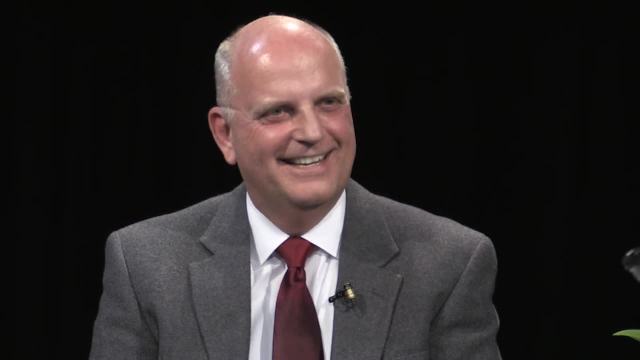 Isn't there something you can do? And I said, well, no, there really isn't an orchid that gets you high? And there really wasn't. But I was just undereducated because about 15 years ago, a friend of mine who was working, 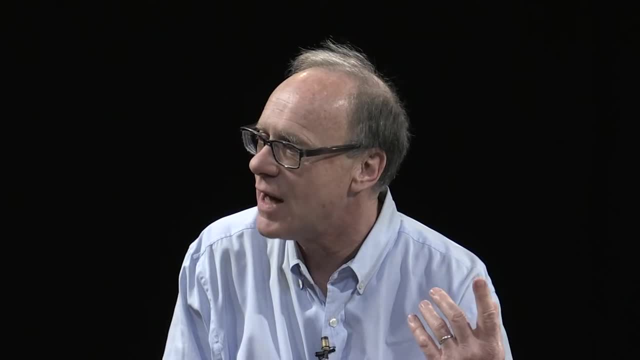 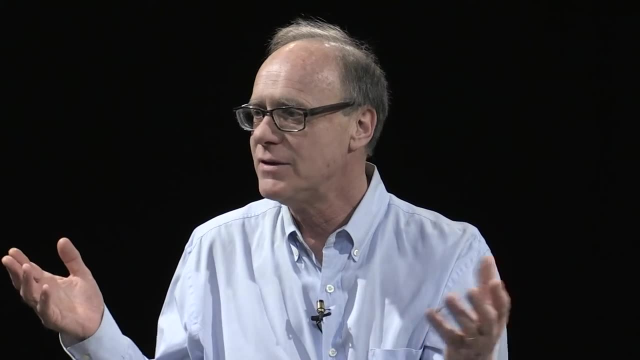 who does social and social anthropology down was down in Mexico And there is indeed a type of rat tail on sitting which we don't have here tonight. that is hallucinogenic, is a strong hallucinogenic. Oh, how funny. 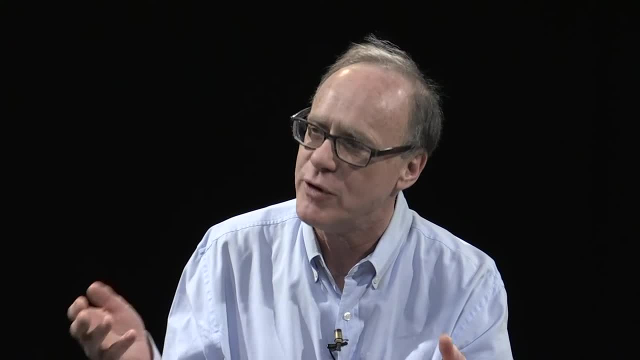 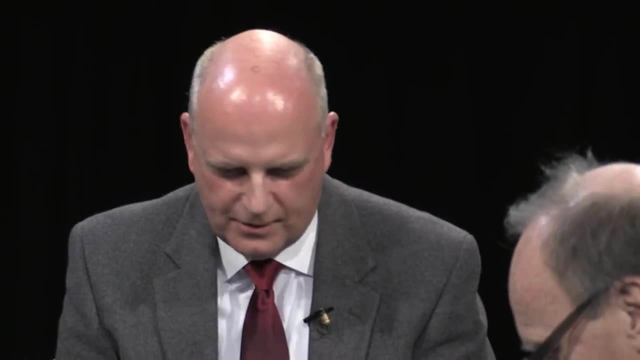 But because all that's been lost, pretty much all that pre-Columbian knowledge has been lost to us. We just don't know that anymore, what's going on. So it's very, very interesting. We have you know we're moving through stuff here. 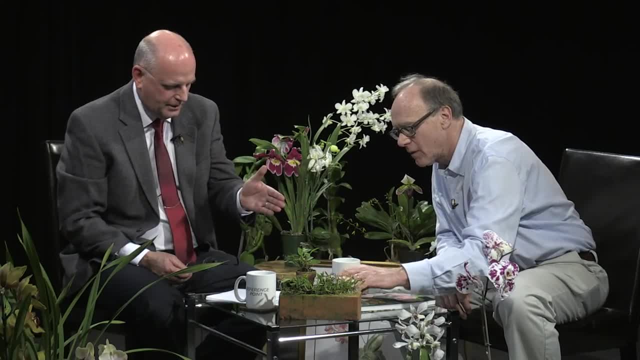 This has been fascinating. I want to talk a little bit about the book that's on the table there and this fantastic print that you have here too. So let's touch on the book a little bit. This is your book, correct? 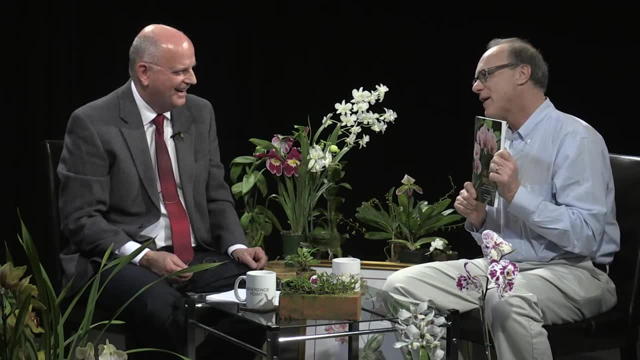 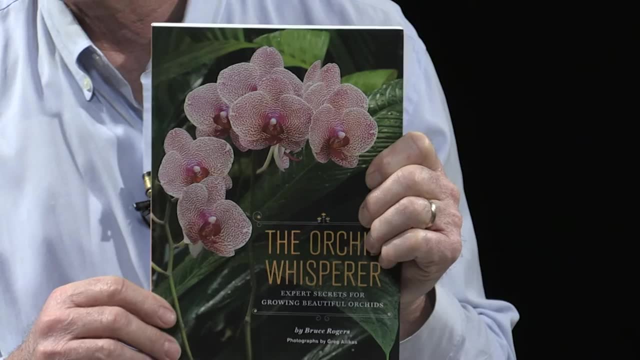 This is my book. I have to admit, this is my book: The Orchid Whisperer. I told you the little story about it being named. I thought they were calling me up to do a book on Sabrellia breeding, but no. 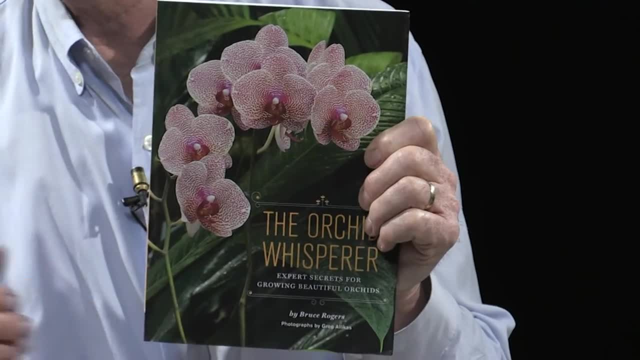 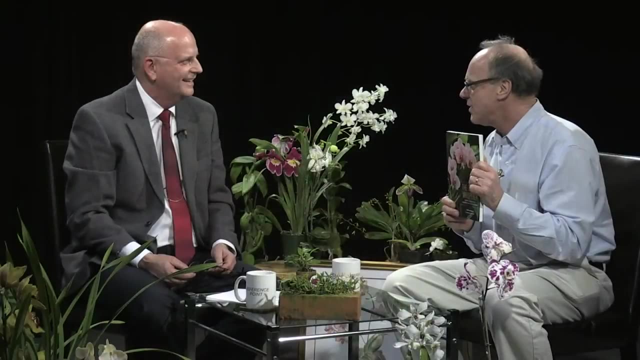 they decided that wouldn't sell any books And they had been on TV a lot. and you TV guys have been very nice and called me the Orchid Whisperer since the moniker came out And my wife kicked me so hard. she says: 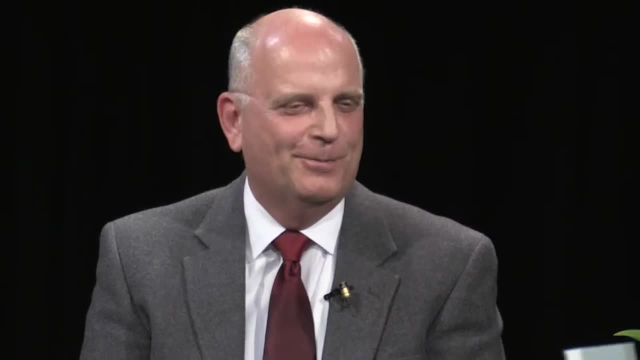 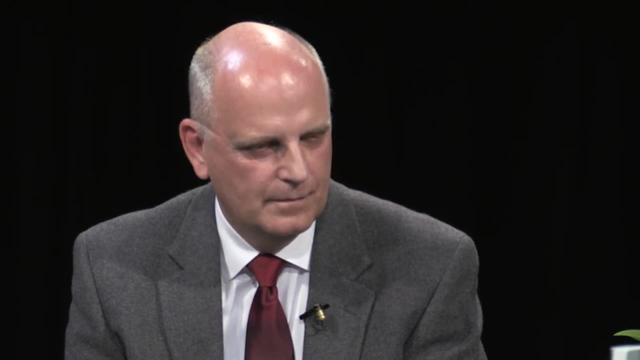 you just let them call you whatever they want, Bring home a check As long as they like the book. And then the book. I worked with Chronicle on this book and Chronicle was wonderful. We're in the seventh printing. It's the best-selling orchid book in the world. 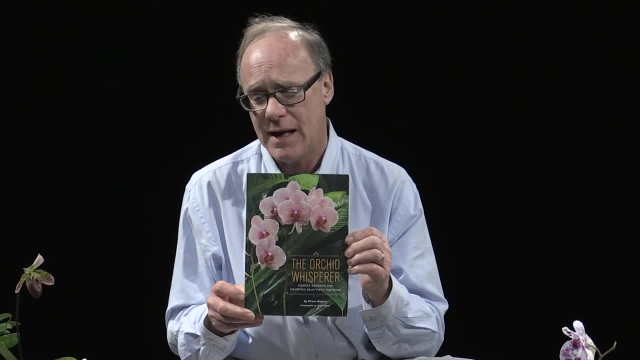 as far as I know, Certainly the best-selling orchid book in the world over last Christmas And it's currently sold out. but as soon as we get some copies we're gonna get you a nice copy for your wife, And in this book you do what. 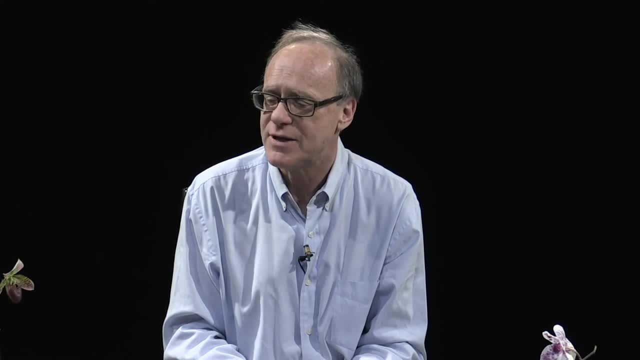 What do you talk about? Well, that's just, it's a general beginner's book and it's just talking about that. I take the different groups much like we're doing here tonight. David, I talk about the different groups. 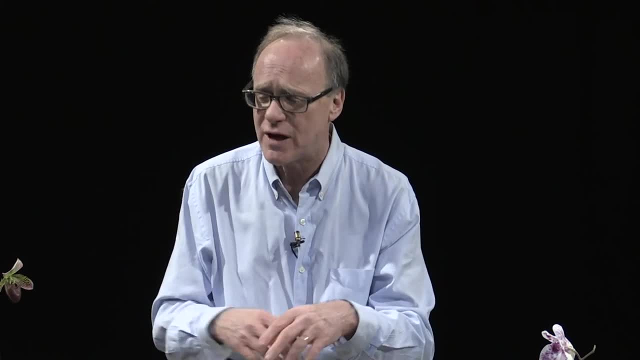 where they grow, how should you grow them? but it's meant for the whole country, so I have to be kind of general, Got it. It's kind of a general thing, but then there's a lot of new things happening that people don't know about. 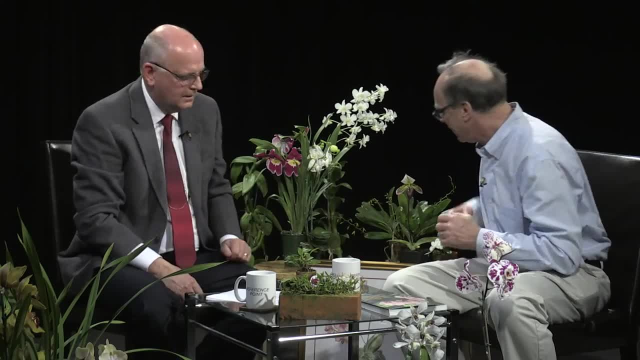 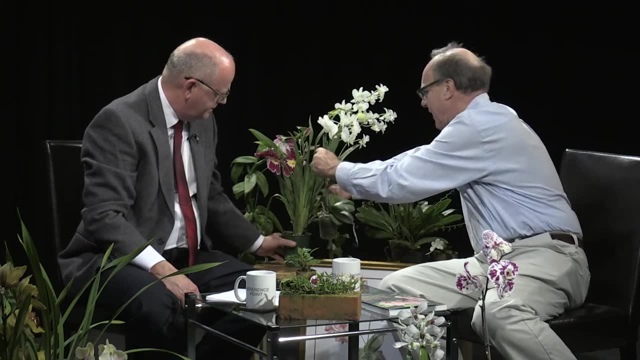 and I'm gonna talk about one of those right now too. I'm gonna take this orchid right here. You hold that orchid over here. I'm gonna pull this right off the thing because I want to see this. This is called a Phalaenopsis. 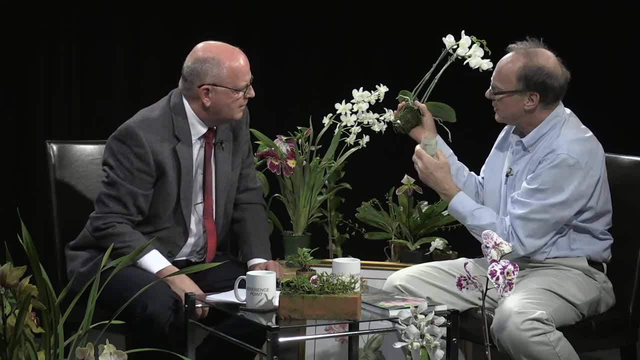 and this is kind of interesting. You see how this is growing, not in bark, but it's growing in this moss. Oh, yes, Now most of the Phalaenopsis growing today, if you look at this type, except for this one. 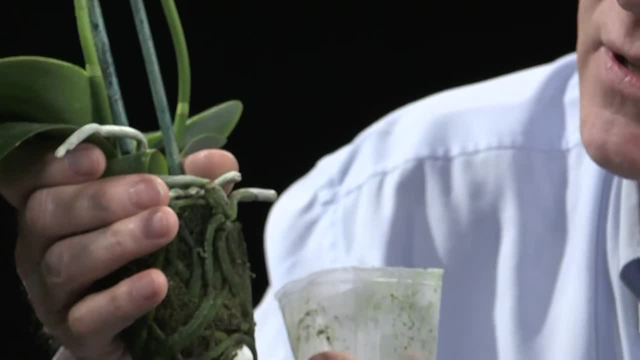 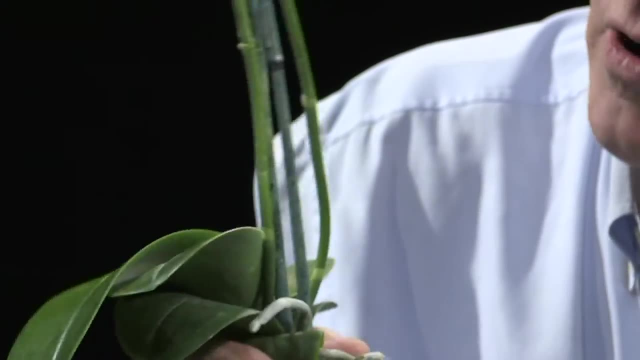 but that one is. they grow in this moss At the big box stores, Trader Joe's. it's growing in this moss. Now, this moss you have to be careful of in terms of watering, because you actually have to water by weight. 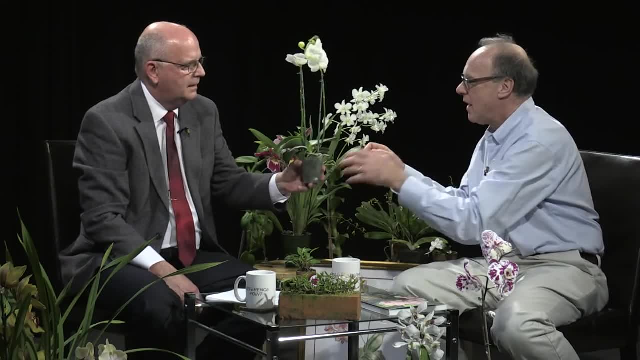 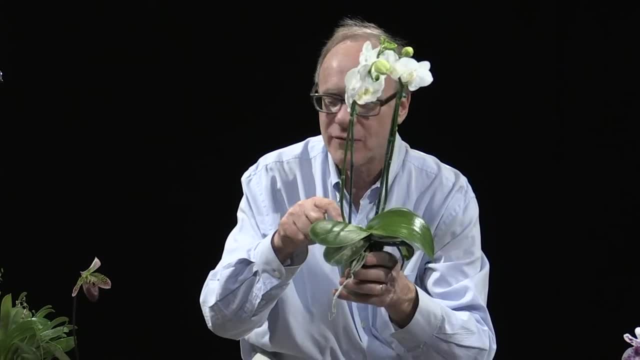 By weight, Because it's watered now and you feel how it's heavy. Yeah, Now, what makes this sphagnum moss different? is that because it's sphagnum moss, instead of drying from the top down like everything in the world, dries. 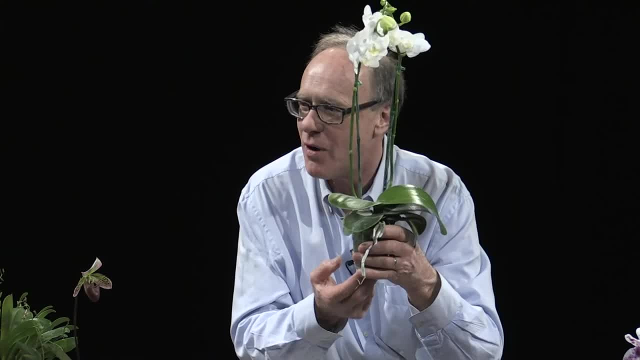 it's like: oh, everything dries from the top down. This sphagnum moss dries from the bottom up because the capillary action of the moss, Oh interesting. And so when you buy this orchid and you get it home, 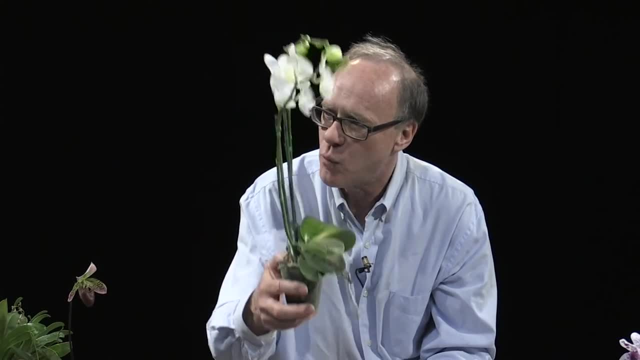 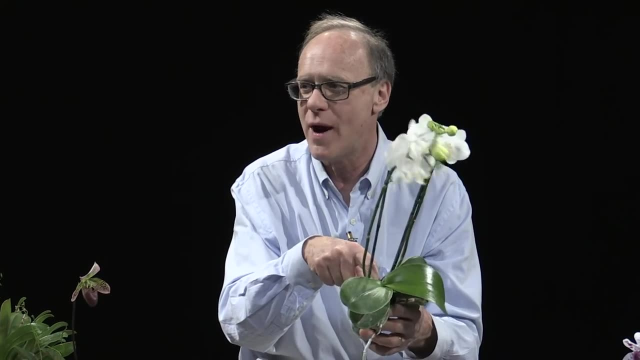 the best thing to do is to bring it to your sink and water it once, and that weight should determine that it has been watered, Because if you rely on looking at the top of the pot, it's saying, oh, it's still wet on top. 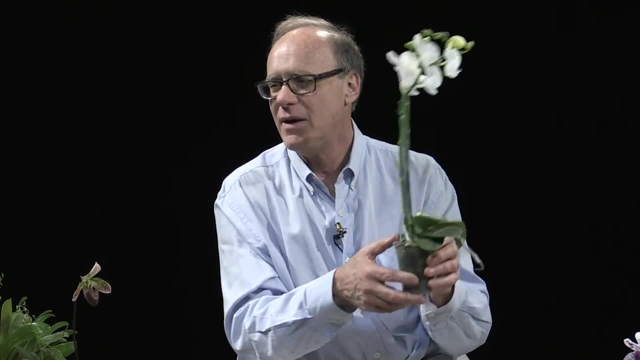 Yeah, Well, that might be true, but the whole bottom might be bone dry. That doesn't mean this can do anything down there. Exactly, You really want to water by weight. And what about this print? Oh, this is a lovely print. 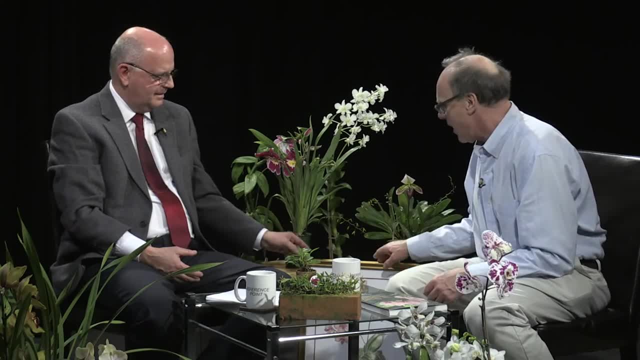 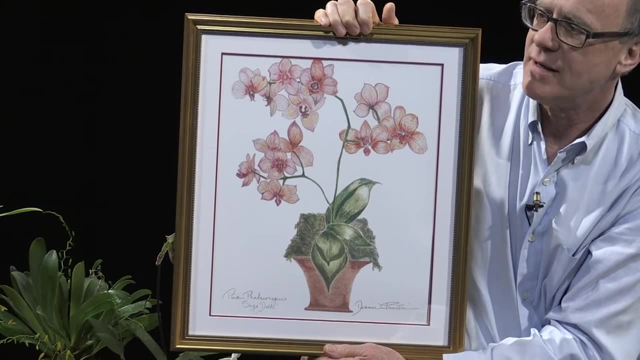 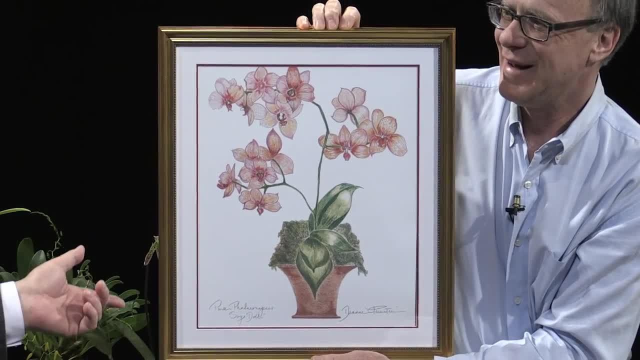 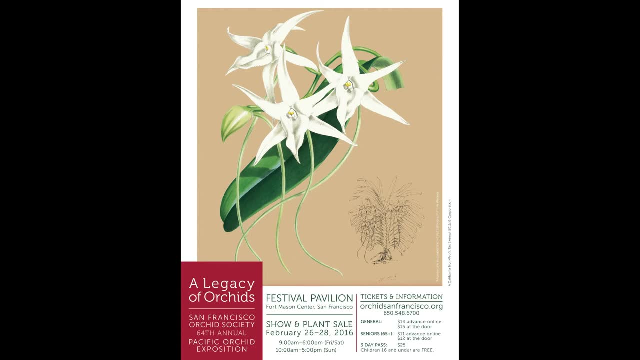 Tell me again The orchid show is when It is a 28th. Do you have it written down, David? Yeah, David knows You'll tell— February 26th through 28th in San Francisco at Fort Mason. 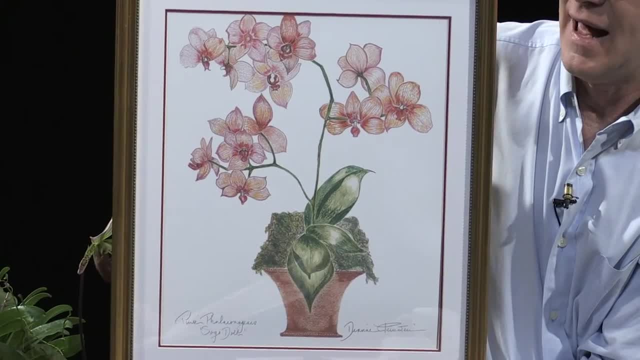 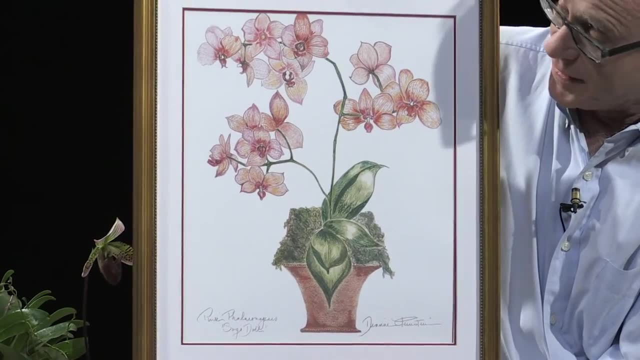 Yes, And this every day, all day long. And as you're walking, you'll see a little table where there's some very interesting things being offered. There's things like this painting. This is Dianne Feinstein. She paints, she paints these and she has a print made. 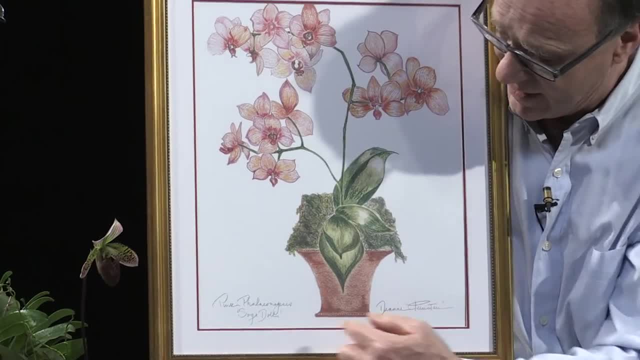 And then she hands her … signs it. I'm there when she hands she actually hand signs it, hand signs it and hand labels the print. And these are very hard to find. These are kind of a neat thing to have from our dear 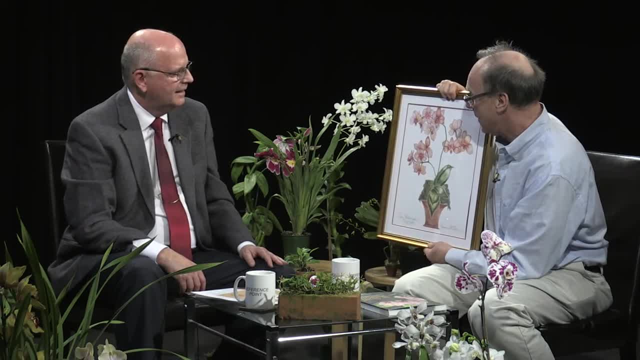 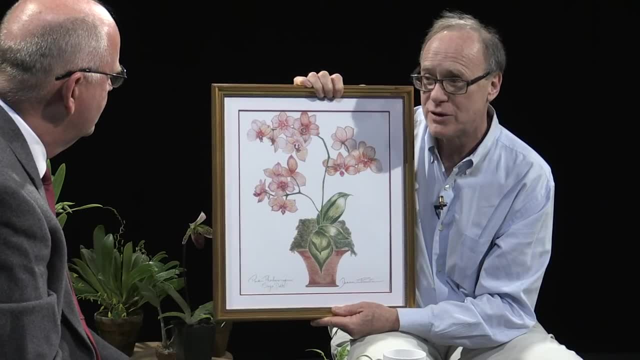 Senator Feinstein, And just to let you know they, I've seen these go anywhere from thousands and thousands and thousands of dollars to hundreds of dollars, And the Orchid Show is one of the few places you can actually find it for just a few hundred dollars rather than thousands Now is. 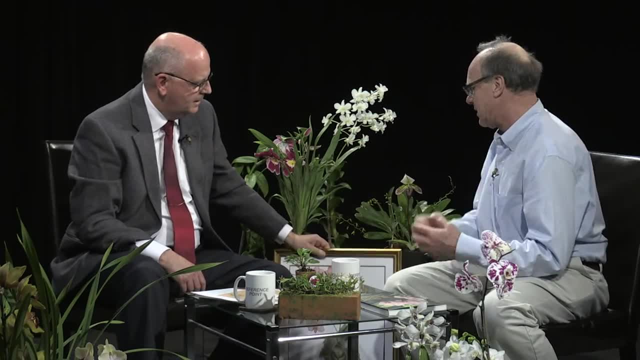 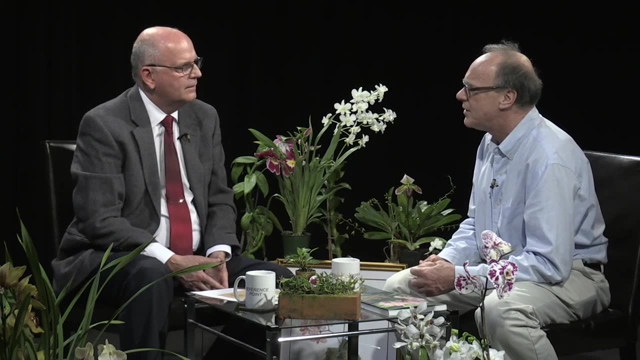 the Orchid Show an annual event. It is Every year. this is we've had tons of them under our belt by now, And this is probably at Fort Mason And it's a very large venue And it's ideal for us. 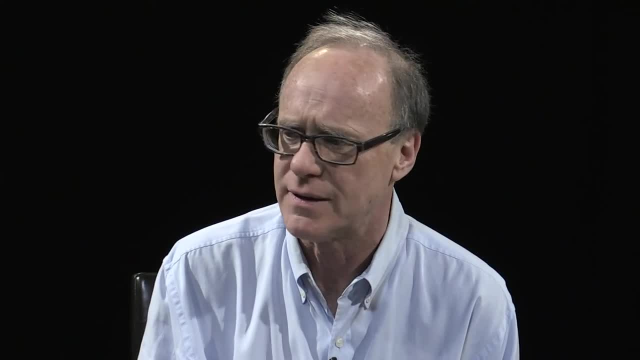 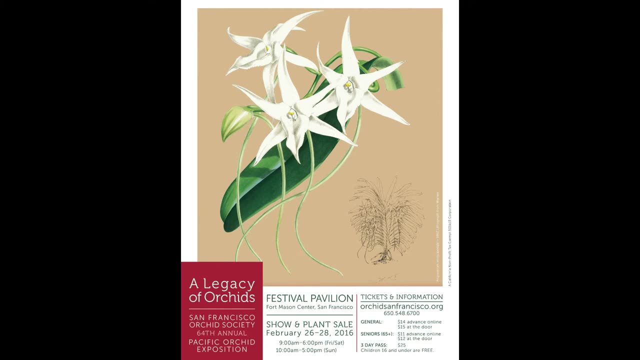 because we get a lot of, a lot of people in there, a lot of people there selling work. According to the flyer, which I think we have an image of that we can put on the screen here, the show is from 9 am to 6 pm on Friday and Saturday and from 10 am to 5 pm on Sunday, And it's 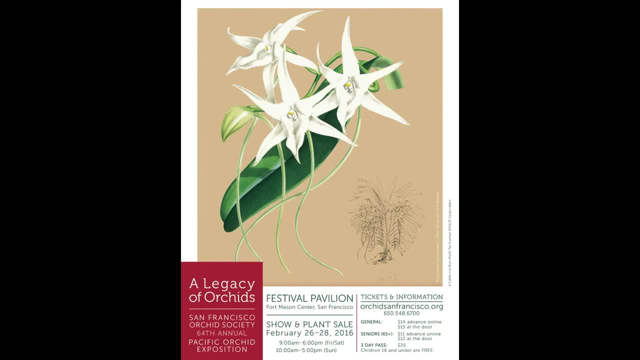 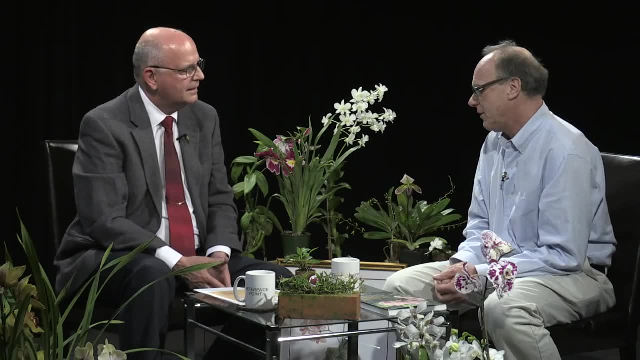 sponsored by the what is it? San Francisco Orchid Society, which is a non-profit organization. Yes, that's the show. It's a society I belong to. It's very strong. We're very lucky. It's one of it's the oldest. 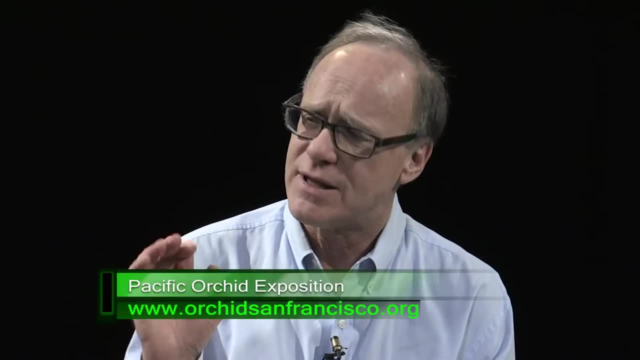 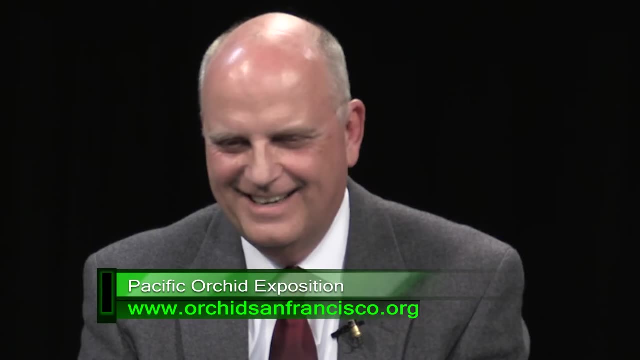 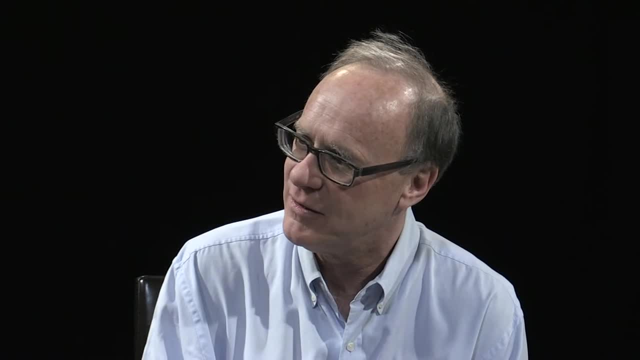 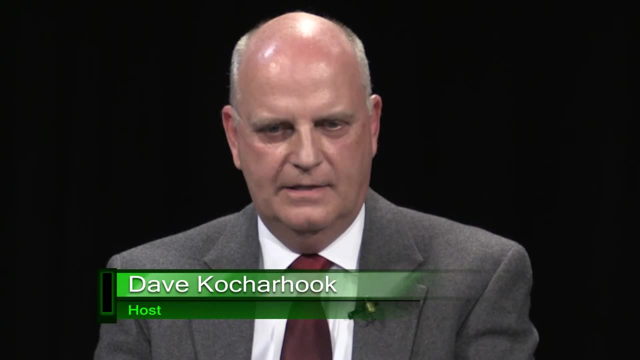 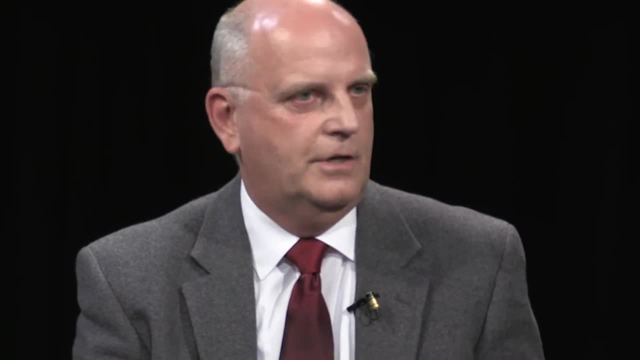 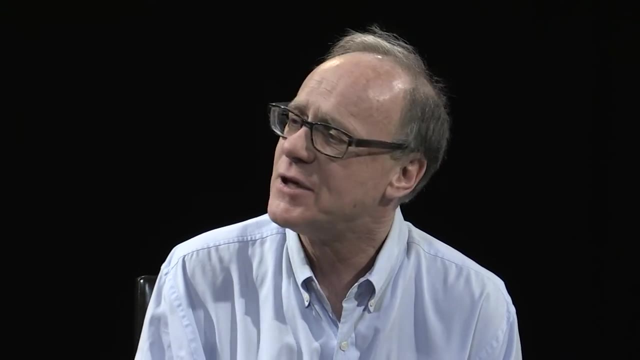 a pot like this, because some people- there's a lot of high density housing here in the Bay Area, So you might have a patio or something and maybe a flower bed that you could grow. Oh, absolutely, You plant these in a fine bark mixture and you can have the whole. I've 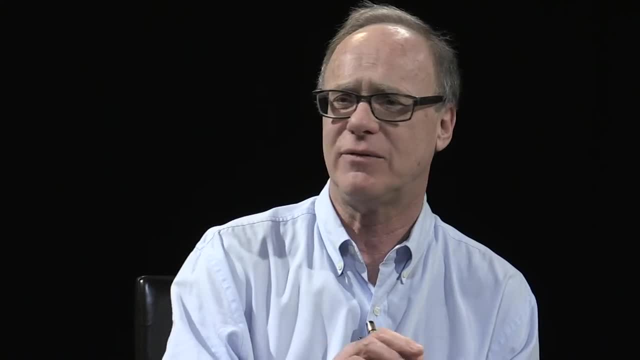 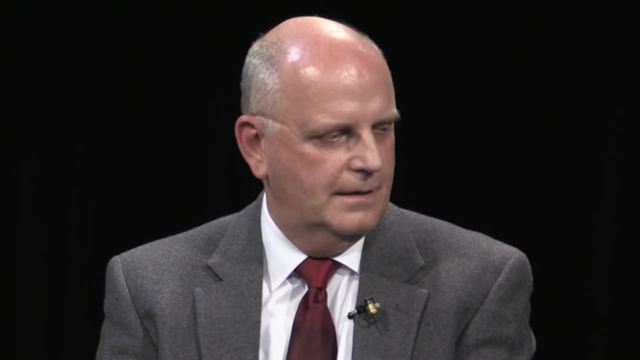 seen hedges. there's hedges of these in Santa Clara. You walk down driveways. they grow them on, on trees even They really, and and actually on tree ferns will grow a lot of orchids. This, for example, this little which I can give to you as a little gift. 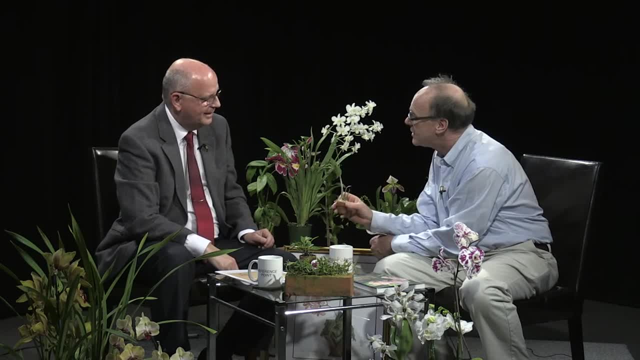 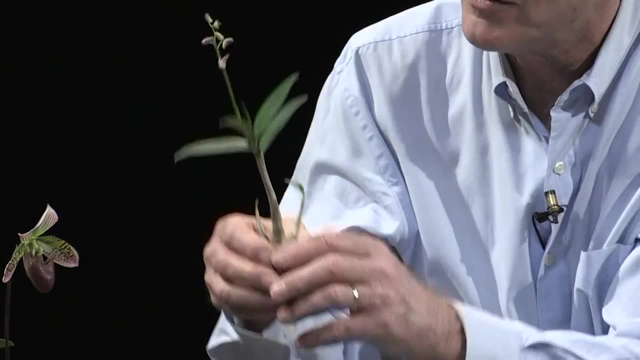 This is a little Dendrobium kinganum from Australia. It's from Australia, just like a, just like a eucalyptus tree. It can grow outside here, just like our eucalyptus can, And this you can actually put into a tree fern. You know those little holes in the tree. 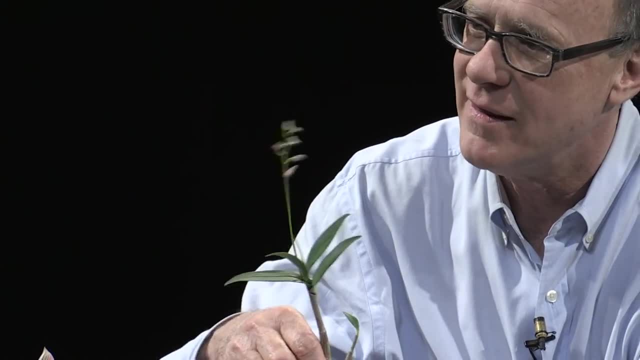 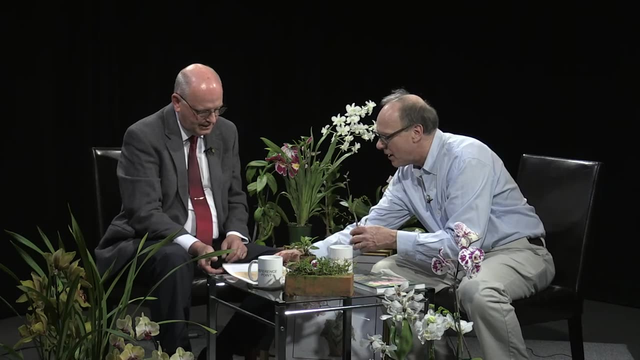 fern, Just stick this little baby right in one of those little holes and it'll grow right in there. It'll grow in there. It'll completely take over the tree, fern. And oh, one thing: I actually got to speak up too. they wanted me to say about: on about. this wonderful orchid show is on Saturday. 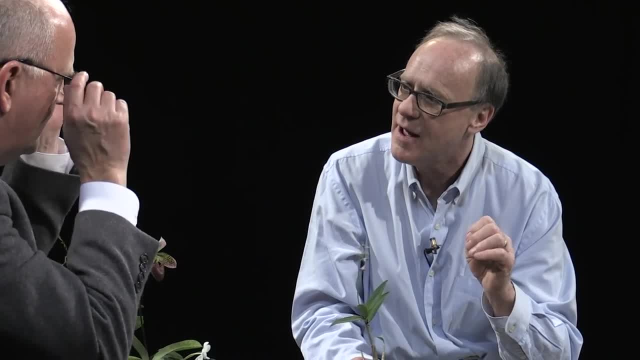 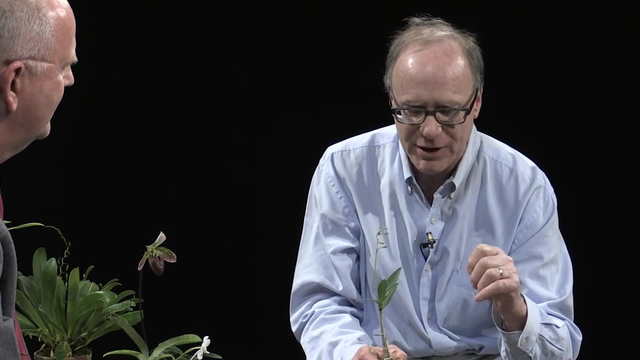 we're doing something new this year. We're having a young person's day on Saturday, Half price if you're under 30. on Saturday, There'll be a great rock and roll band called the Right Siders playing there. Oh okay. 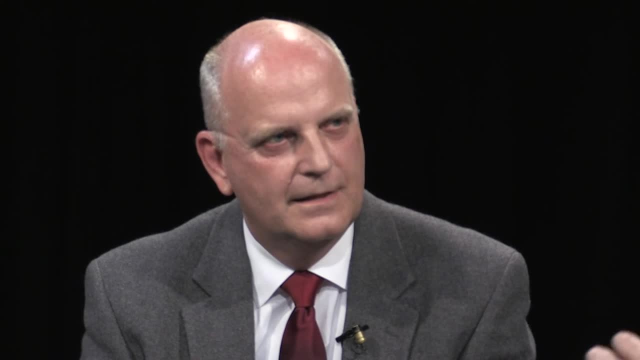 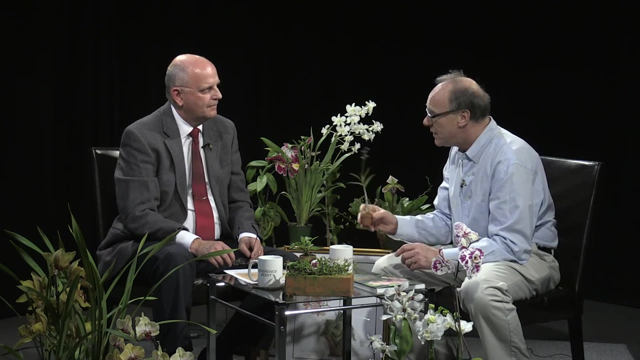 And it should be just a lot of fun for everybody, Because it is a young hobby, Because when you travel you can go out there and find them. if you go to Mexico, you can find them wherever you go. And it's a wonderful hobby to have. And most, most men are, you know. 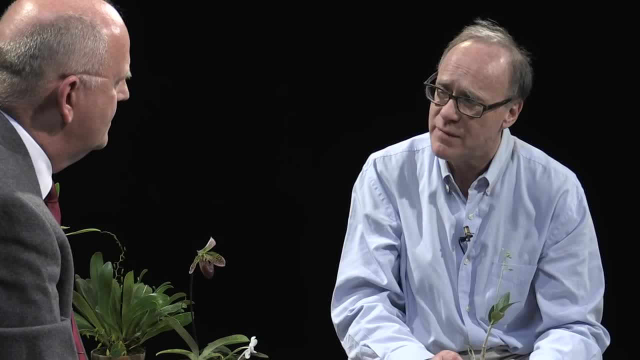 the hobby's pretty much split up between men and women. For as many men as I do for women, Nice, Which is kind of interesting. That is cool. It's not a totally sexist kind of thing, But it's kind of neat too to think about that, Because if you are traveling, whether 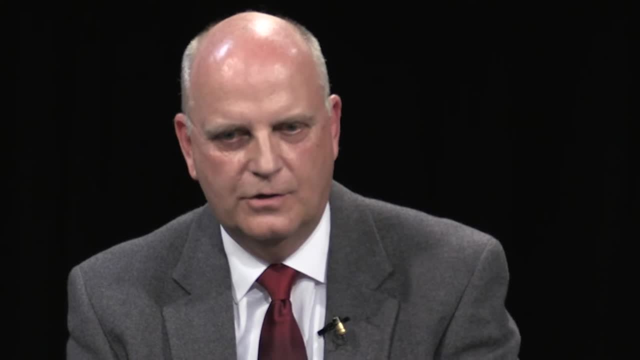 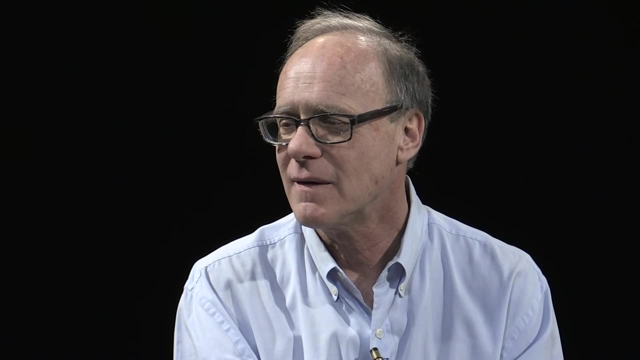 you're going to South America, or whether you're going to Europe or you're going to Asia and you're going to go out and you want to do some hiking or whatever. you have the opportunity and you can really discover phenomenal beauty, which I think is absolutely fabulous. 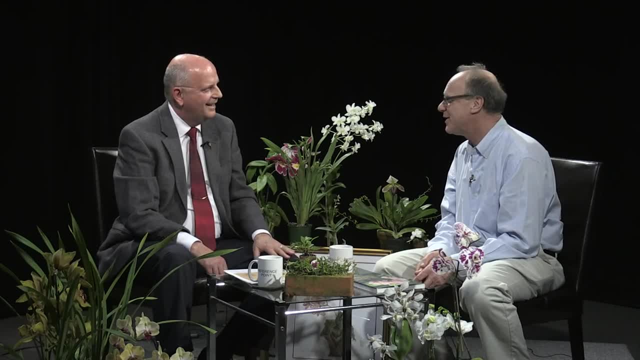 Yes, you really can. And when it gets you out there, you're seeing everything. You're seeing the orchids, but then you're also seeing the birds and the bees and the butterflies. Exactly, And all that comes with it- Exactly. 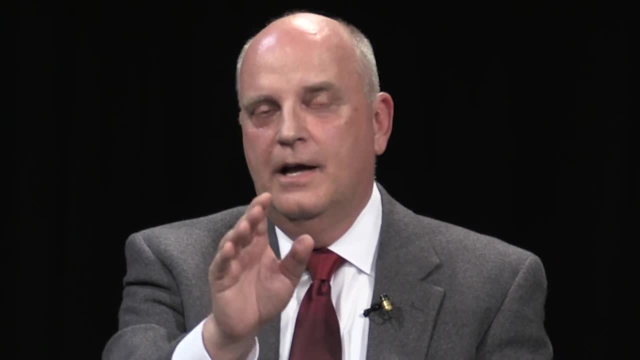 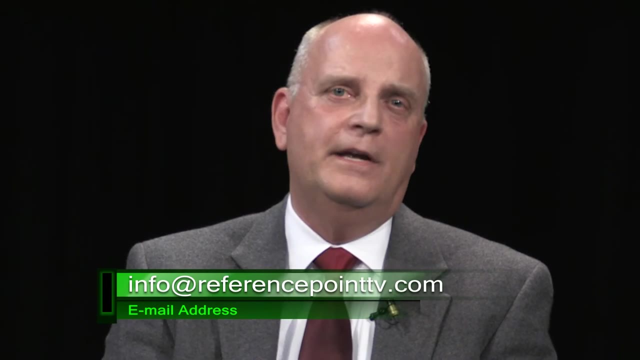 All that Mother Nature gives us Exactly. Well, Bruce, this has been fantastic. I want to remind the folks: if you have any questions about what we've talked about here, about orchids, about the book, about the show coming up at the end of February, send us a query at info at referencepointtvcom and we'll 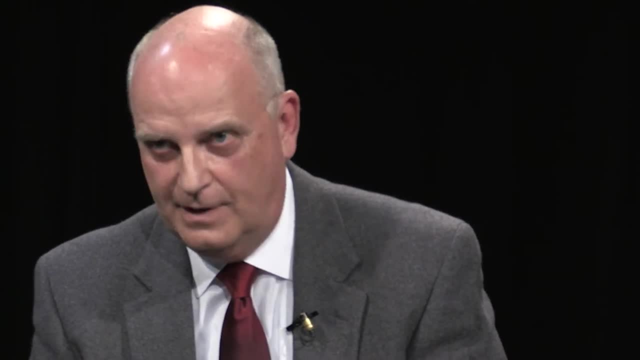 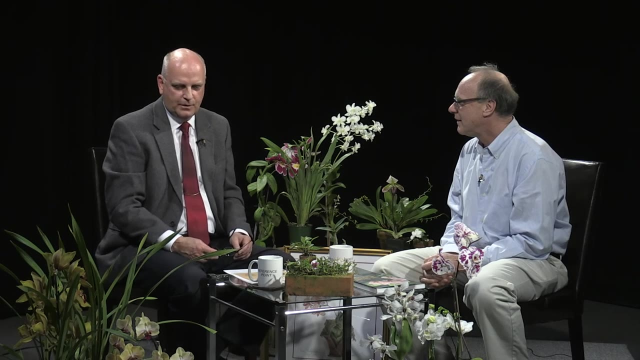 get it to the right party. Bruce, this has been fantastic. I greatly appreciate that you came. The pleasure's mine. I had a lot of fun, Not just yourself being here, but bringing so many fantastic and beautiful examples of the sort of orchids that we here in the Bay Area actually could grow.